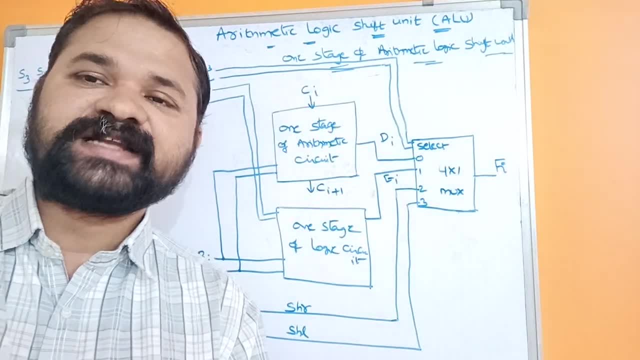 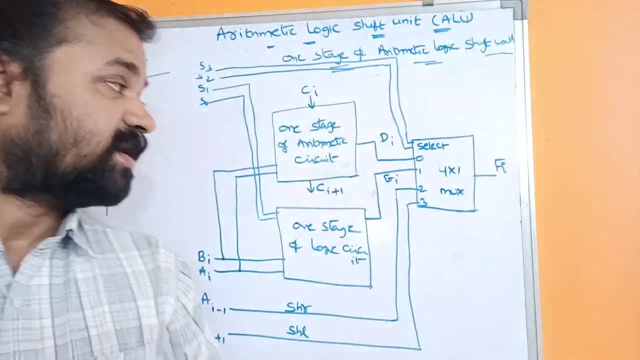 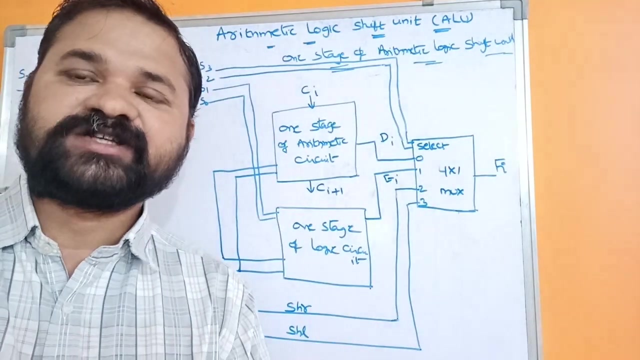 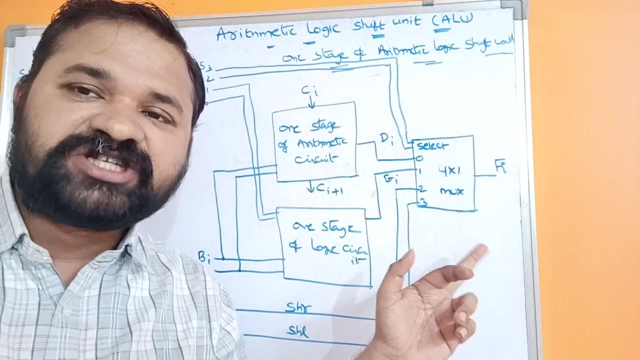 shift micro operations implementation. That is nothing but a 4 bit combinational circuit shifter. So three different videos we have seen, Whereas in this concept what we are doing is we are combining all those three hardware implementations, such as arithmetic micro operations hardware implementation, logical micro operations hardware implementation and shift micro operations implementation- into a single circuit. That circuit is called. 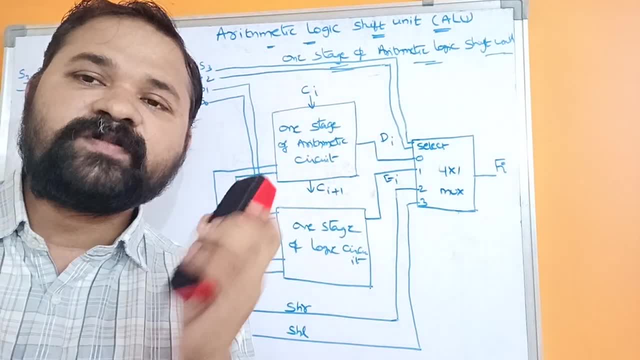 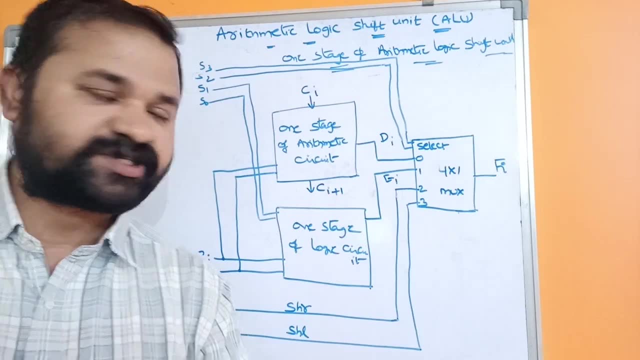 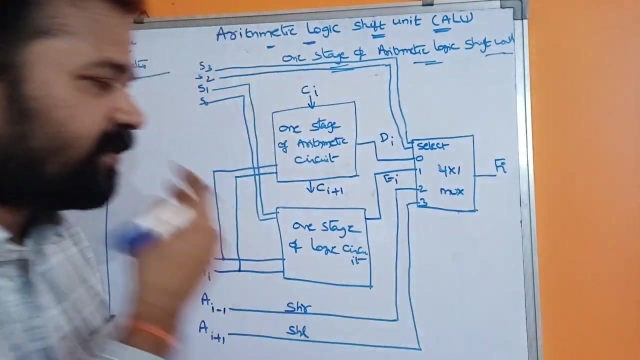 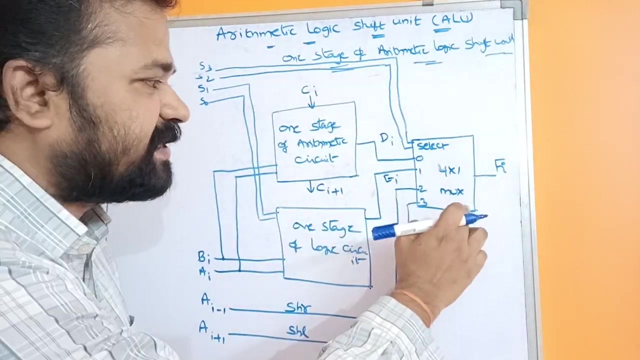 as arithmetic logic shift unit. So arithmetic logic shift unit performs all the arithmetic operations, logic micro operations, as well as shift micro operations. Now let's see this diagram. Here we have a 4 by 1 multiplexer. 4 by 1 multiplexer means we know that it accepts 4 inputs and produces one of the input as the output. So 4 by 1 multiplexer. If it is a 4 by 1 multiplexer, then the selection inputs are 2 by 1 multiplexer. 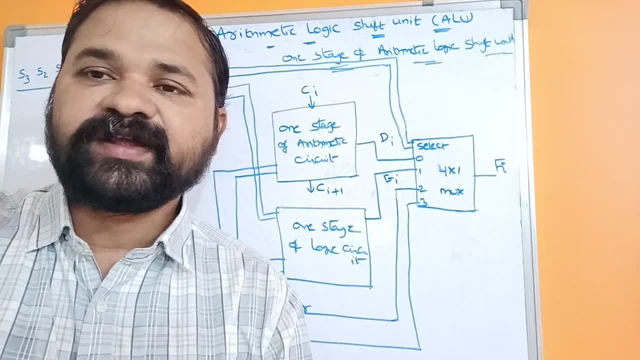 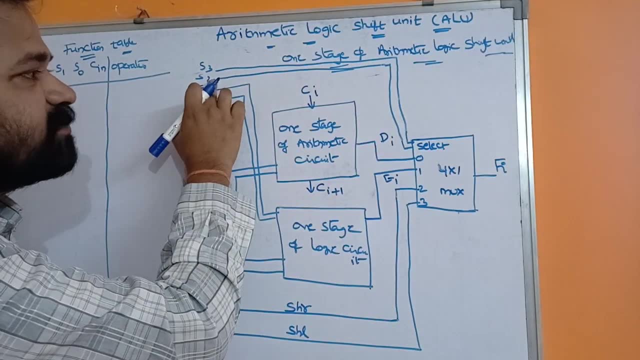 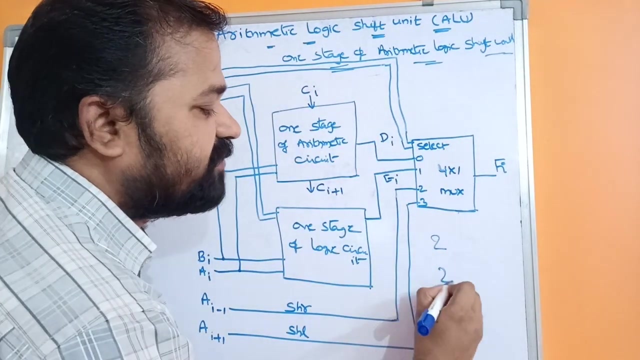 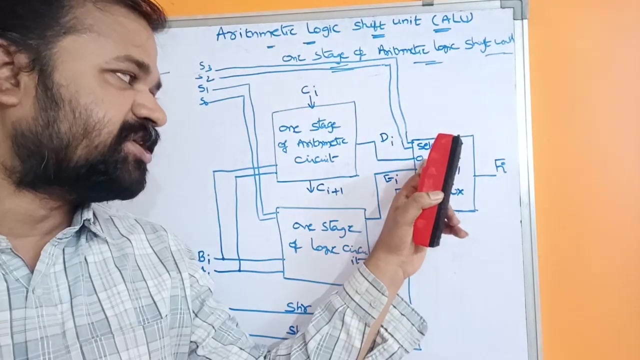 Why? because if there are n selection inputs, then 2 power, n data lines, then 2 power data inputs are needed. So here S3 and S3 are nothing but the selection inputs which are to be applied to the multiplexer. So there are 2 selection inputs are there. So totally we can have 2 power, 2 inputs. So 0, 1,, 2, 3 are nothing but inputs of the multiplexer. Here 0 receives input from the output of the arithmetic circuit. So that is. 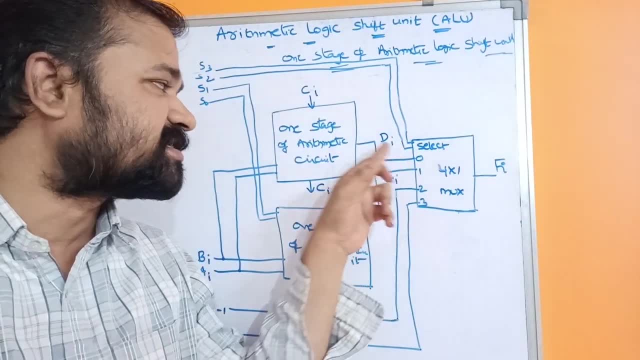 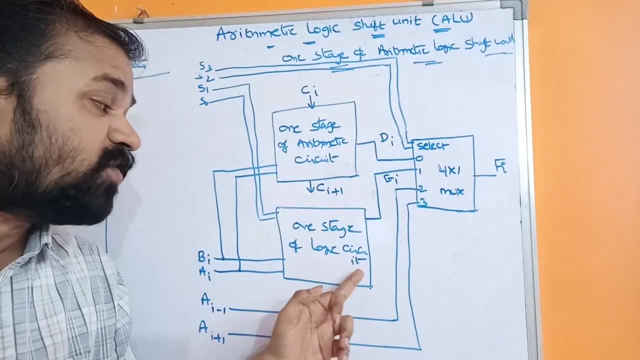 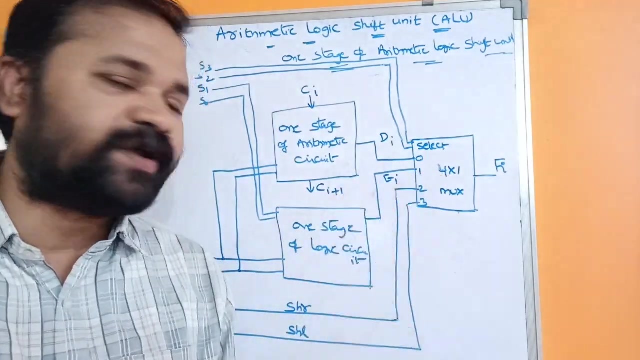 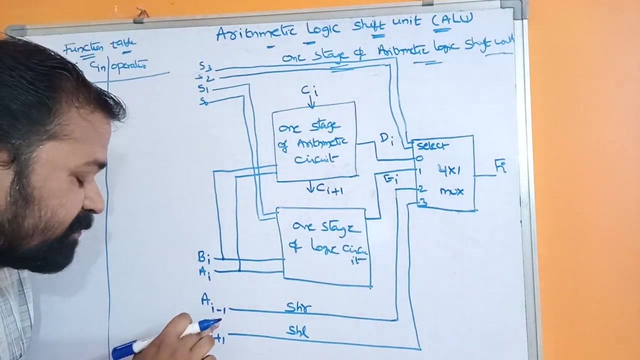 means if we select 0, 0, then it performs arithmetic micro operation. Next 1 input receives data from 1 stage of logic circuit. So 1 input receives data from logical circuit. So if we select 0, 1, then it performs logical micro operations. Next 2 data input receives data from A I minus 1.. Here it is a bit. Here we are using this bit in order to 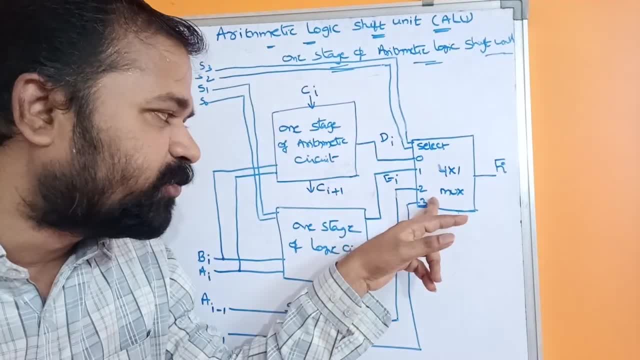 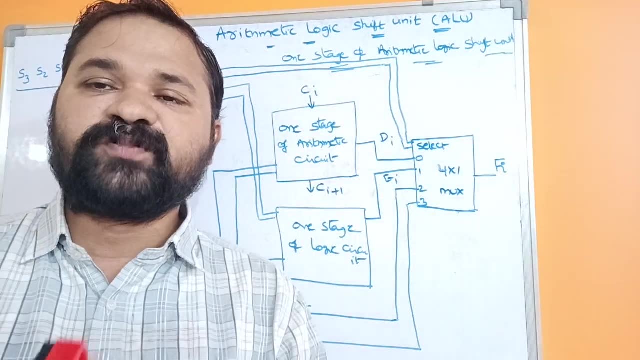 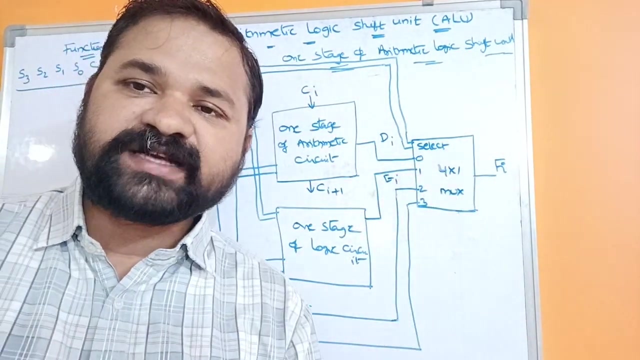 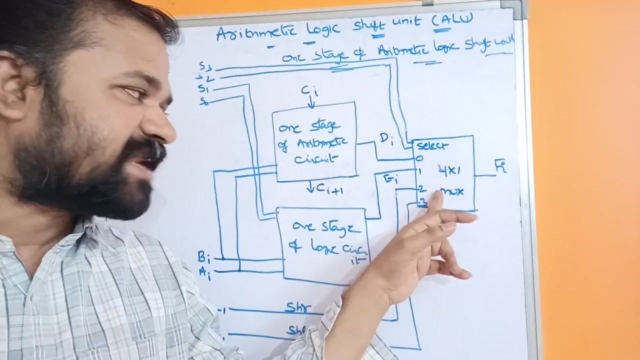 perform shift right operation. Next, 3 input receives data from A, I plus 1, which performs shift left operation. Here the point is very, very simple. Here the multiplexer is accepting 4 inputs. If we select 0, 0, then arithmetic micro operations will be performed. If we select 0, 1, then logical micro operations will be performed. If we select 1, 0, then shift right operation will gets performed. If we select 1, 1. 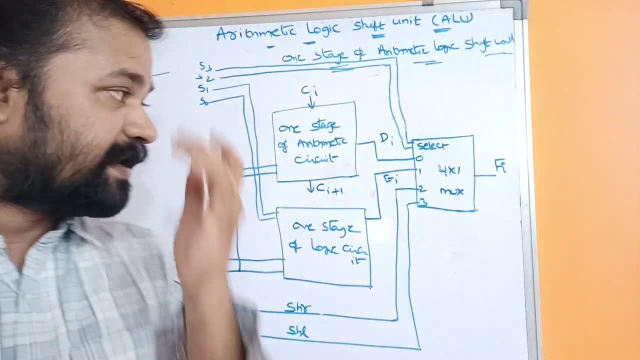 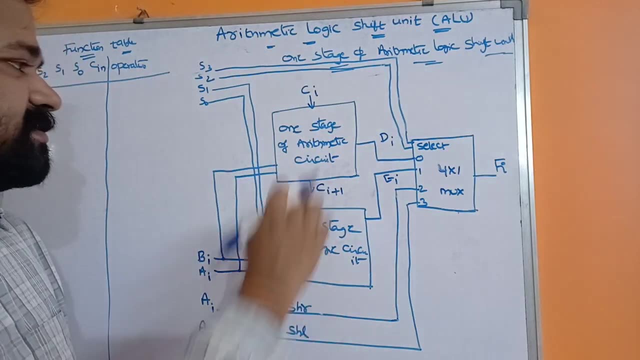 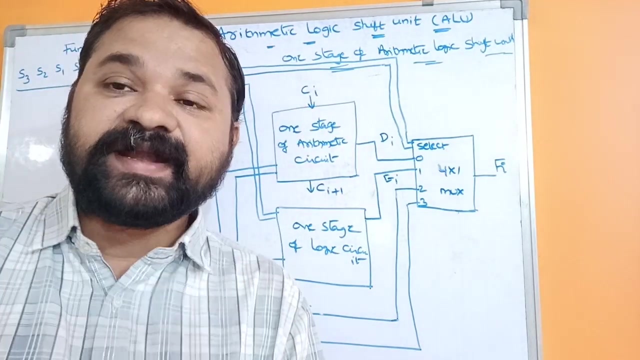 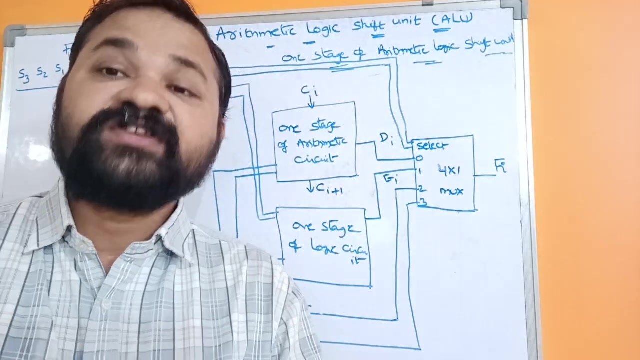 then shift left operation will be performed. Here we are using the selection inputs S3 and S2 in order to control this multiplexer. Now let us see this boxes. So this box is nothing but 1 stage of arithmetic circuit. So already we have seen about arithmetic circuit diagram. So in that diagram, totally we have taken a register, Just we have taken a register which contains 4 bits. So totally 4 bits are taken. A naught: A1, A2, A3, A4, A5, A6, A7, A8,, A9, A10, A11, A11,, A12,, A13, A14, A14, A15, A15, A16,, A17,, A18, A19, A19, A20, A21, A21, A22, A23, A23, A23,, A24,, A24, A24, A25, A25, A26, A26, A27,, A27,, A28,, A29,, A28,, A29, A29. 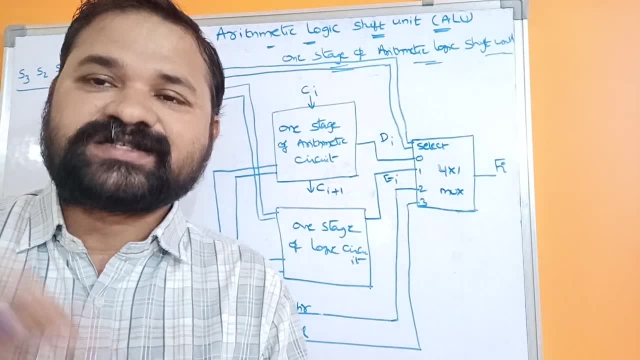 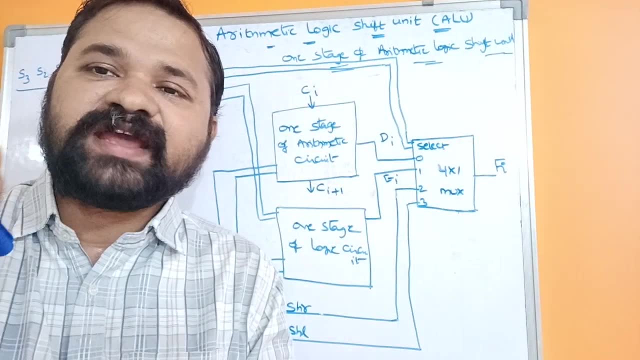 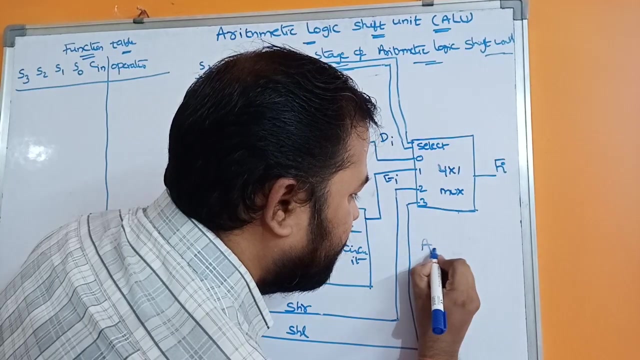 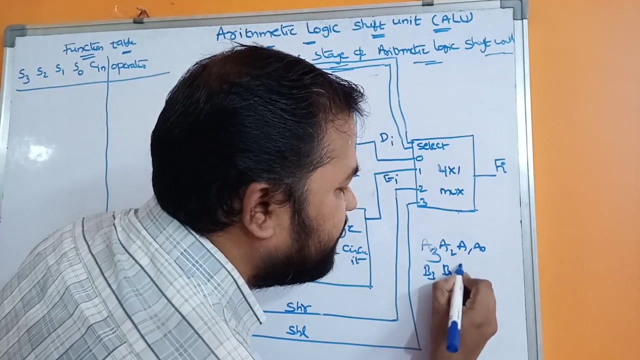 B0, B1, B2, B3 and some carries C0, C1, C2, C3, like that. But in this circuit what we have taken is we have taken only the single bit Only, we have taken only the first bit. Let the first register content is like this: A0, A3, A2, A1, A0.. Let the second register content is B3, B2, B1, B0.. Let the initial carry is C0. So here we have taken only A0, B1, B2, B3. 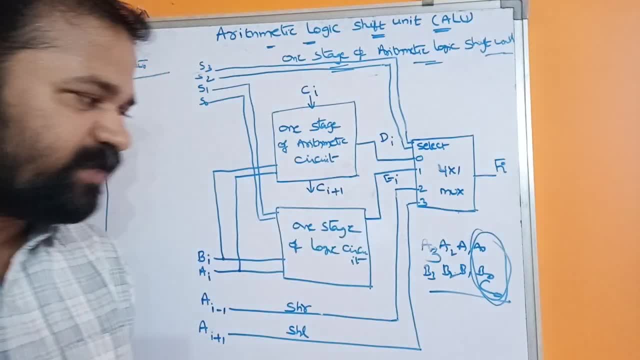 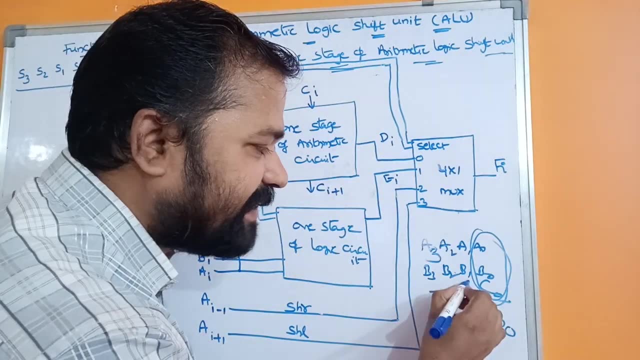 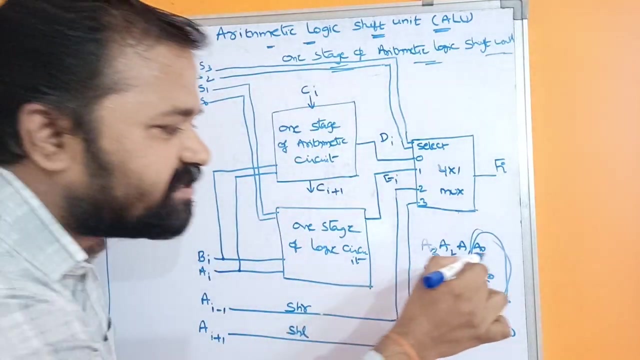 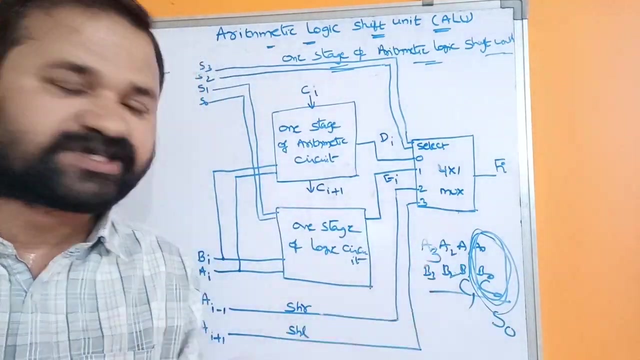 B0 and C0.. Let us assume that we are performing some addition operation. So after performing addition we may get some sum value as well as we will get some carry. So let the carry is C1.. So let us see this diagram. This is nothing but one stage of an arithmetic circuit which performs addition operation or any operation on only the corresponding bits A0, B0, C0, A1, B1, C1. like that. Here CI is nothing but input carry to the arithmetic circuit. So this is C0. 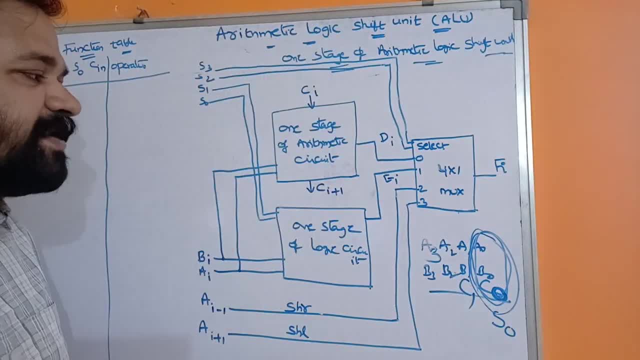 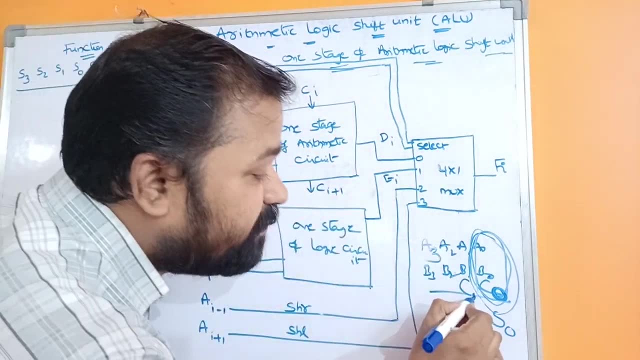 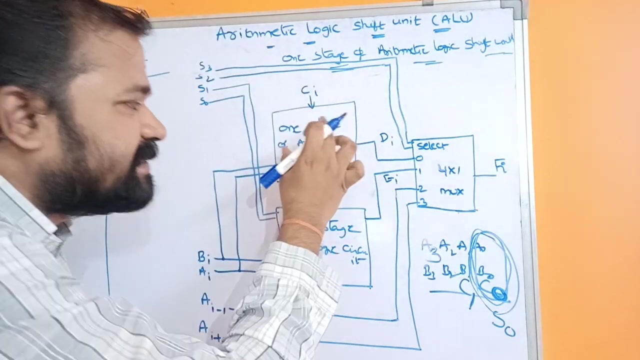 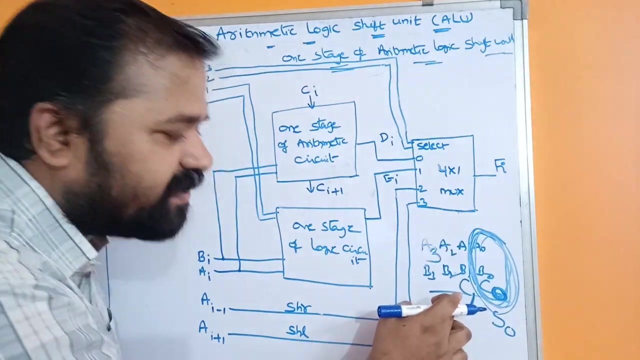 C0 is nothing but here the input carry. So if you perform any arithmetic operation then we will get some output carry. Here the output carry is nothing but CI plus 1.. That CI plus 1 will be passed as input to the next stage of the arithmetic circuit. So what is the next stage of the arithmetic circuit? Here this arithmetic circuit is performing operations are A0, B0, C0. So if we add these three numbers we will get some carry, So that carry value will be passed to the next stage of the arithmetic circuit. So the next: 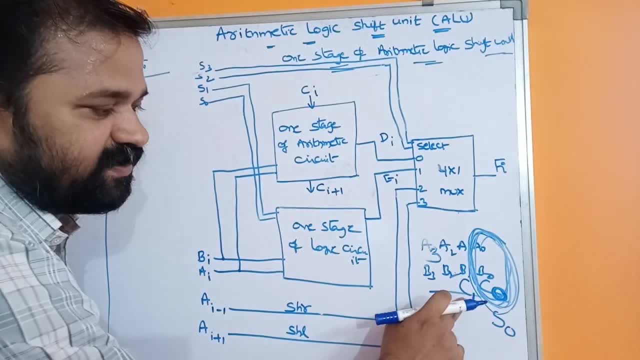 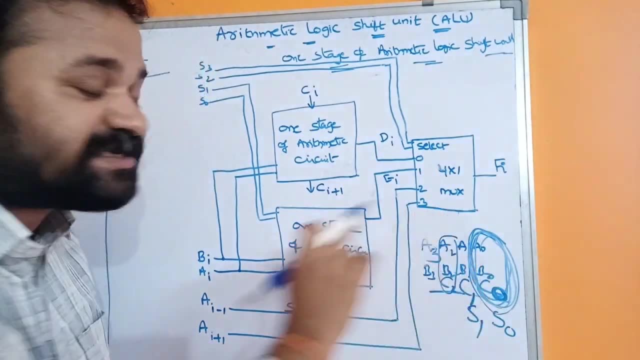 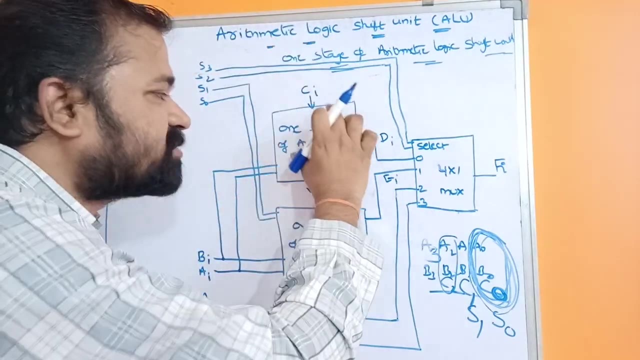 stage will perform operations on A1, B1, C1.. Then we will get some sum value. Next we will get some carry, So that carry value will be passed as input to the next stage of the arithmetic circuit. So if you want to perform operations on four bits, then we have to repeat this one for four times. 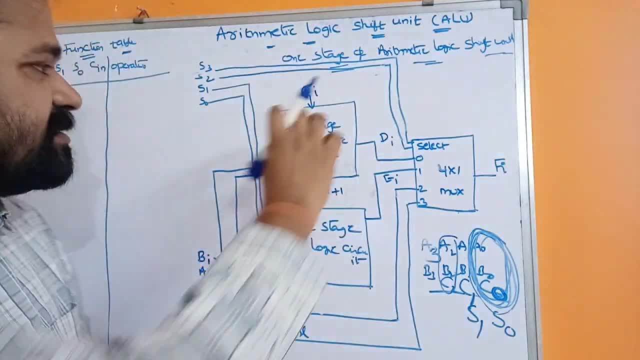 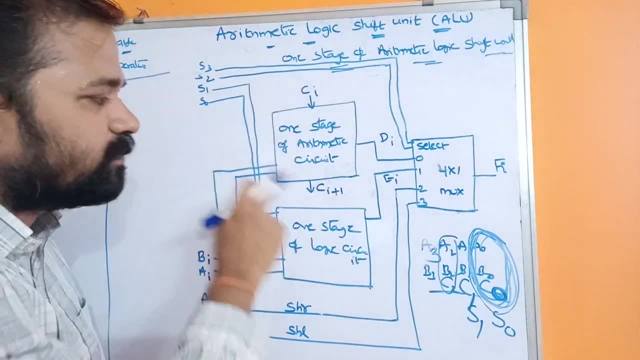 We have to repeat this stage for four times. So this is nothing but arithmetic circuit. So very, very simple. So here arithmetic circuit is accepting some input- carry- And it is producing some output carry- CI plus 1. This will be passed as input to the next stage of. 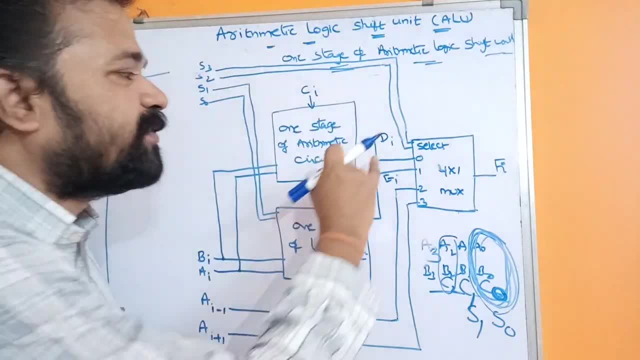 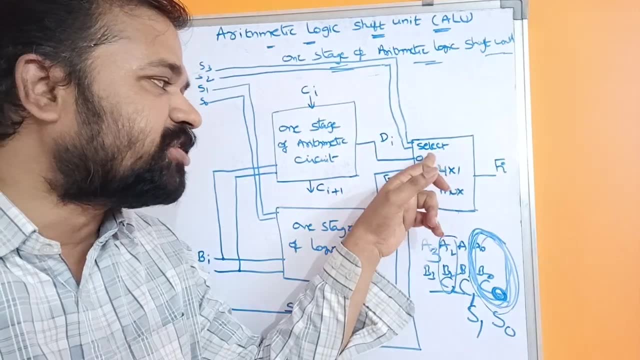 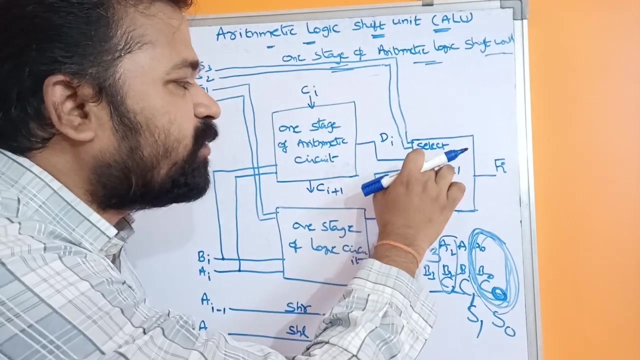 the arithmetic circuit And the output of the arithmetic circuit is DI. The DI is passed as input to the zero input of the multiplexer. So if we select 0, 0, then what will happen? This zero input output will be produced. So what is the zero input? Zero input is getting data from. 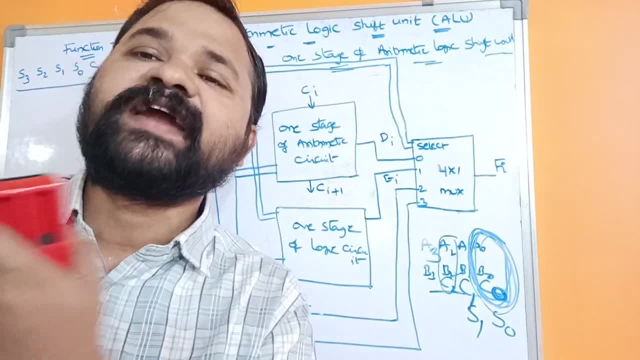 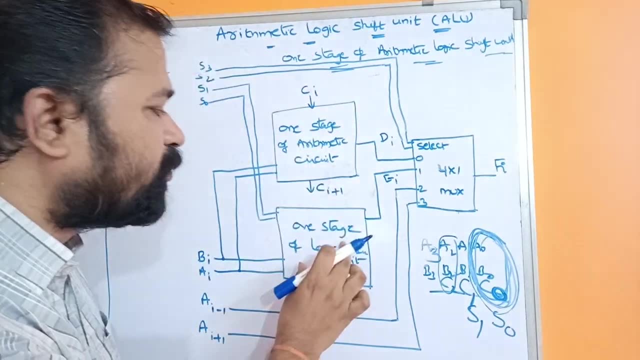 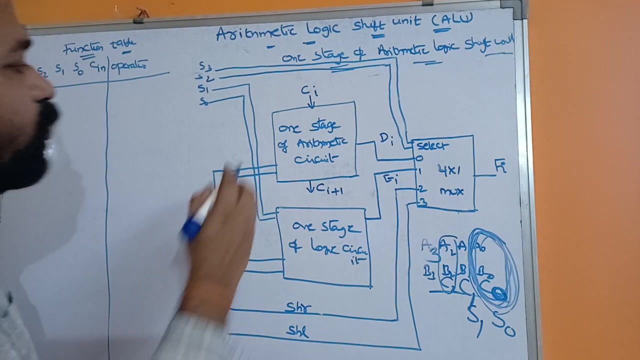 output of the arithmetic circuit. So arithmetic operations will get performed. See this one. This is nothing but one stage of the logic circuit, So the output of here also we are using some selection inputs: S1 and S0.. S1 and S0 controls arithmetic circuit as well as logic. 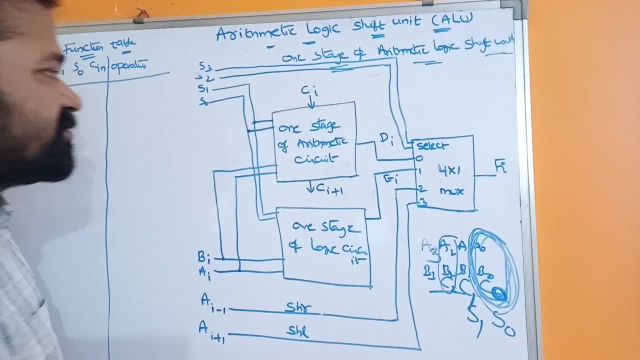 circuit. So this is nothing but S1.. This is nothing but S0.. So S1 and S0 are the selection inputs which are to be applied to the arithmetic circuit as well as logic circuit. So here also the logic based upon the operation of the arithmetic circuit is getting data from the arithmetic circuit. 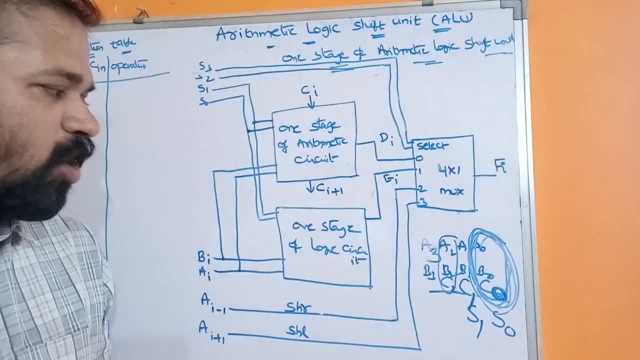 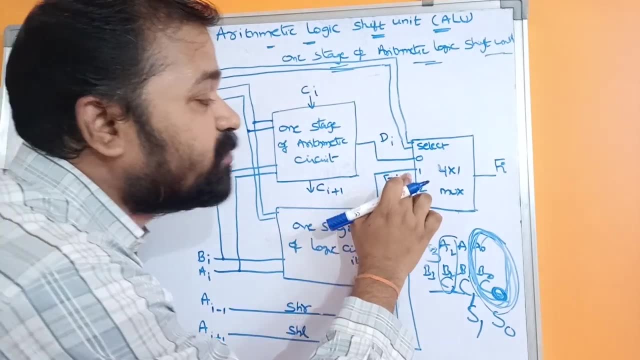 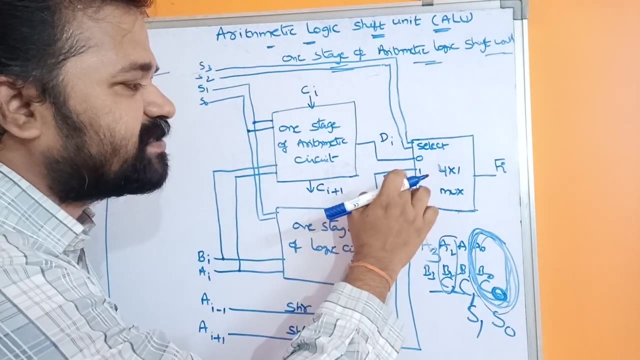 The logic circuit will perform the corresponding operation and it produces the output. That output is denoted by EI, So EI is passed as input to the data input 1 of the multiplexer. So output of the logic circuit is EI, So that EI is passed as input to the input 1 of the multiplexer. Here for the 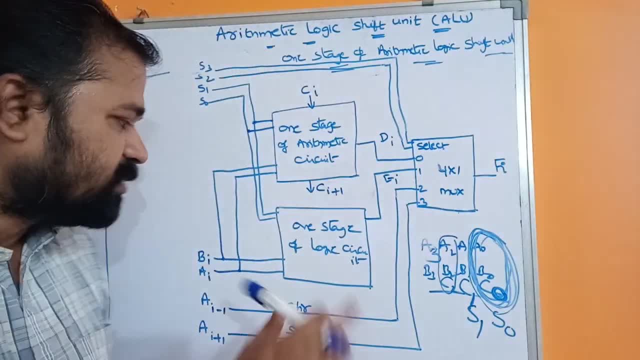 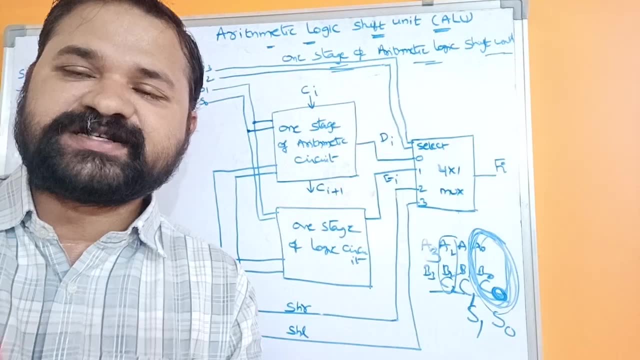 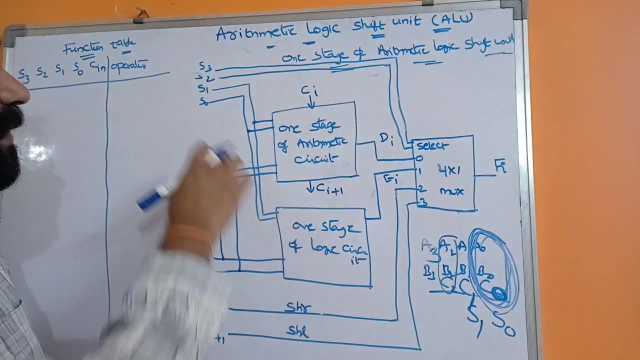 logical circuit. we know that there is no need of any carry, So there is no need to specify any carry for the corresponding logic circuit. We know that we have mainly four logic operations. are there Logic and under operation, R operation, exclusive R operation and complement operation. Those operations are controlled with S1 and S0. 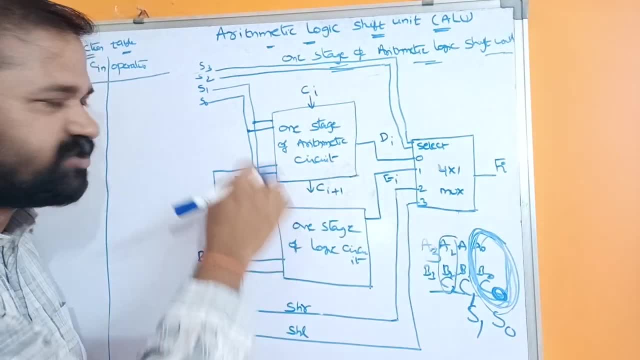 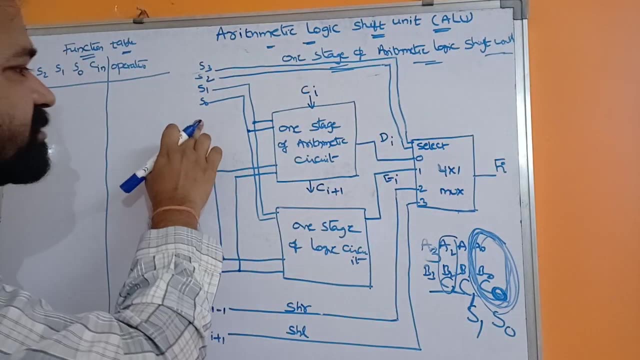 So if S1 and S0 is 0, 0, then perform some under operation. If S1 and S0 is 0, 1, then perform some R operation like that. So here S1 and S0 is controlling arithmetic circuit as well as. 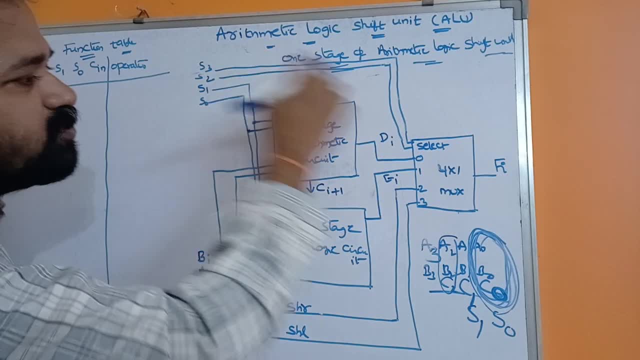 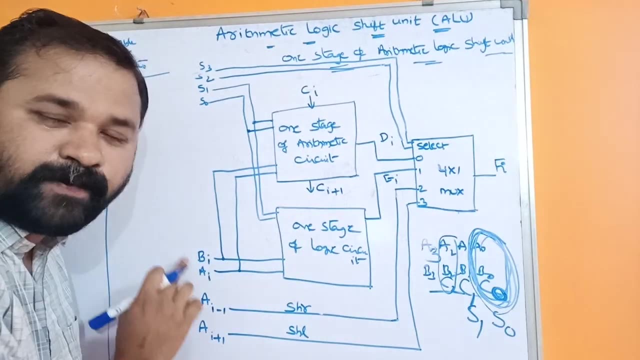 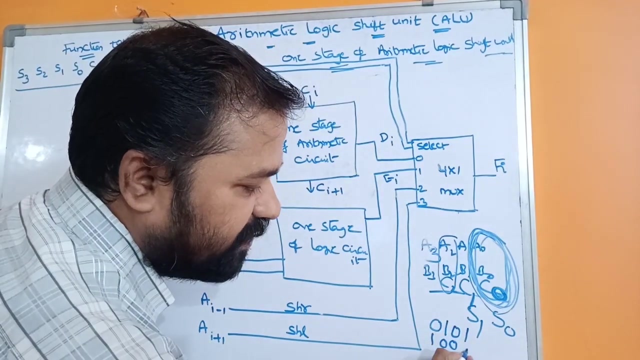 logic circuit, Whereas S3 and S2 selection inputs are controlling the multiplexer. Next, what are AI and BI? AI is nothing but register A bit. BI is nothing but register B bit. If you take this example: 0, 1, 0, 1, 1, 0, 0, 1.. So this is nothing but AI. This is 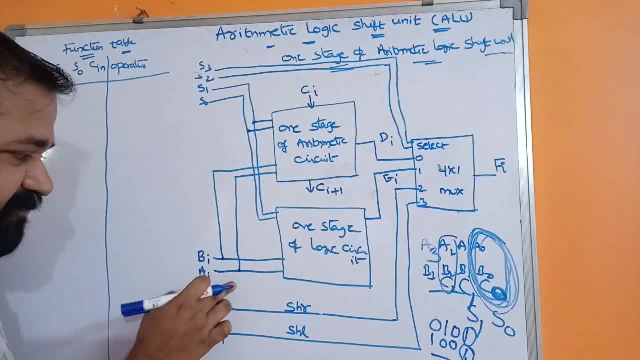 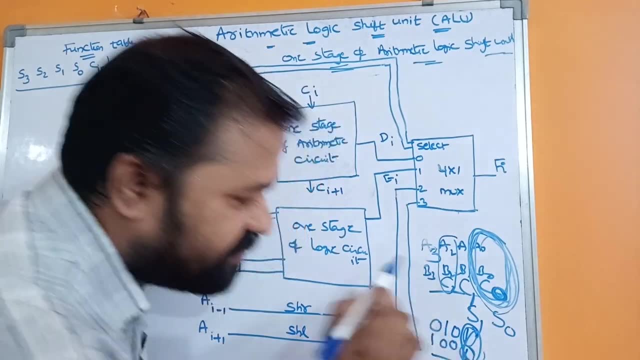 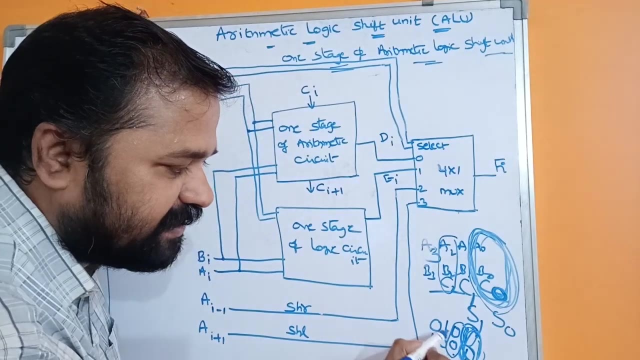 nothing but BI, So A0, B0.. So that information we are passing to logic circuit as well as arithmetic circuit. Here we are passing only these two bits. So once operation is performed on these two bits, Then these two bits will be passed. This 0, 0 will be passed. Next, this 1, 0 will be passed. So 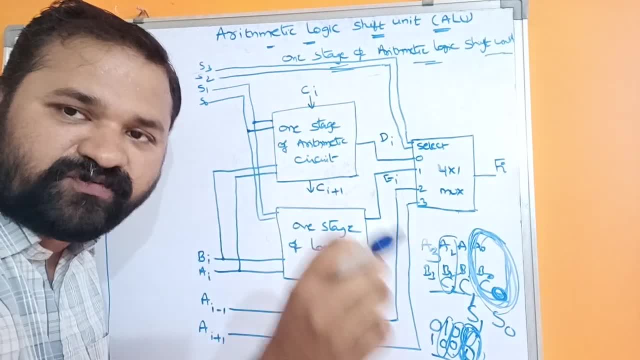 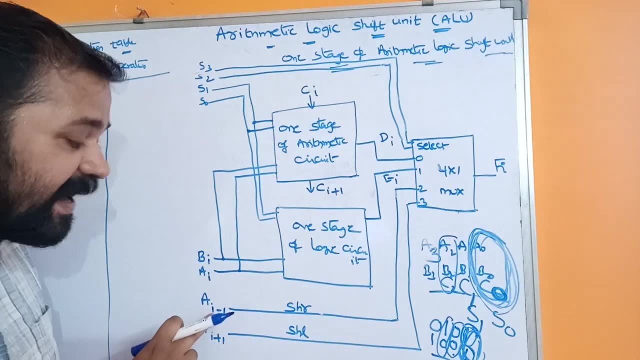 further we are using this one. AI represents one bit of register A. BI represents one bit of register B. Next, AI minus 1.. AI minus 1 represents a bit which is useful in order to perform shift to right operation. Next, AI plus 1 represents a bit which is useful in order to perform shift to. 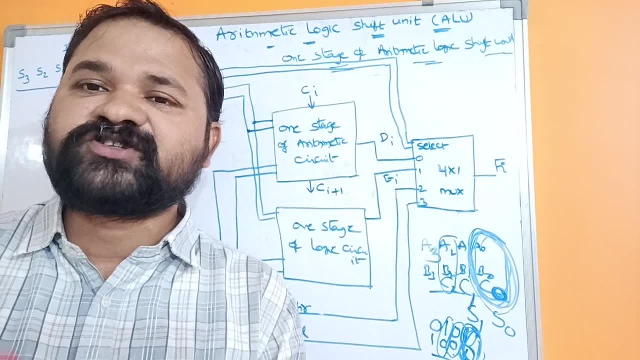 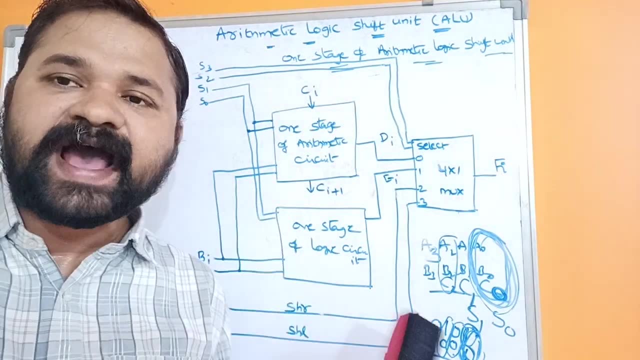 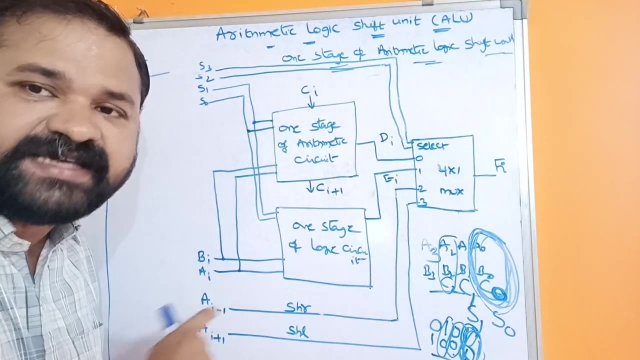 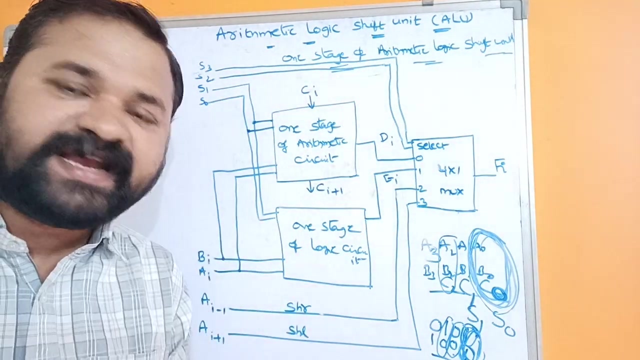 left operation. So here the naming conventions is also very, very simple. A and B are nothing but register content. So we are passing AI and BI as inputs to arithmetic circuit as well as logic circuit. Next, AI minus 1 is a bit which performs shift to right operation. AI plus 1 represents a bit which is needed to perform shift to left. 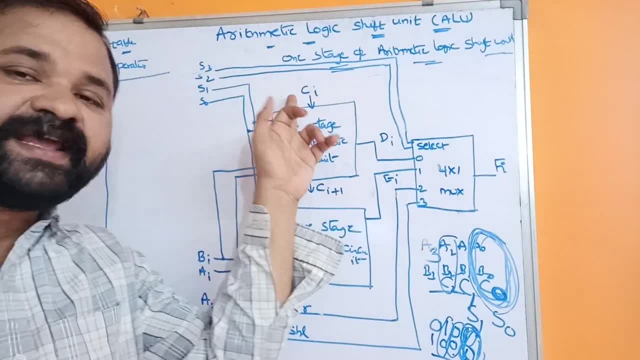 operation, So A is over, B is over Next. CI represents input capital, So AI plus 1 represents a bit which is useful in order to perform shift to right operation. CI plus 1 represents output carry, So CI is over, Next D. 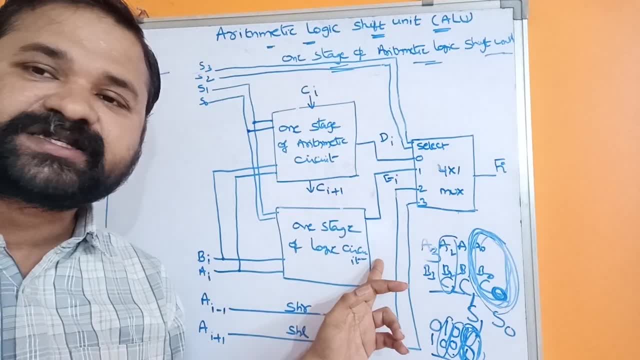 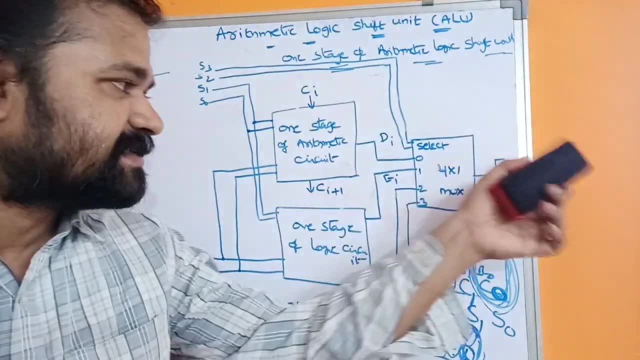 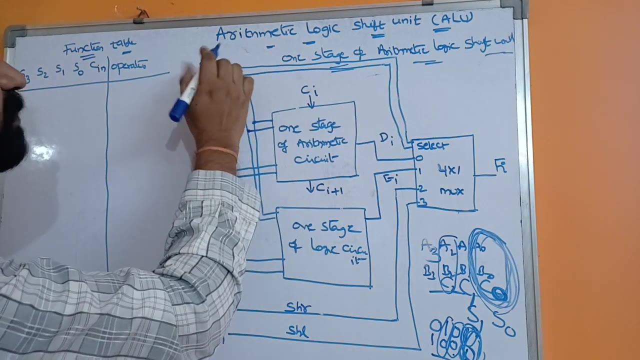 represents output of the arithmetic circuit. E represents output of the logic circuit. F represents the output of the multiplexer. So which operation we are performing? That is nothing but F. Now let us analyze this diagram. If the selection inputs are 0, 0.. Selection inputs means these inputs. If S3 and S2 are 0, 0. Then which? 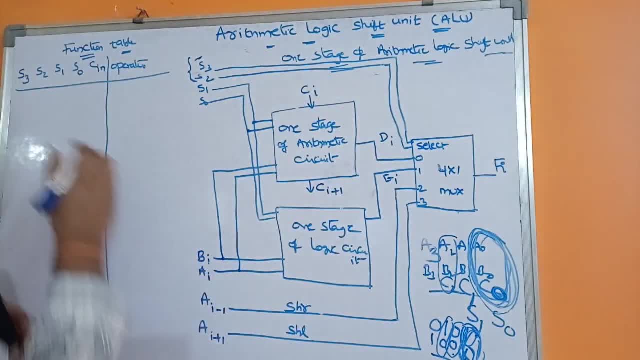 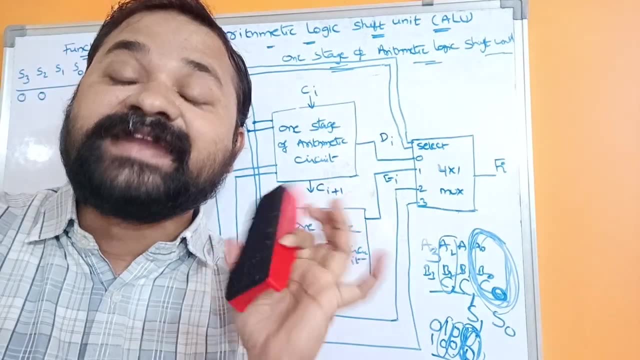 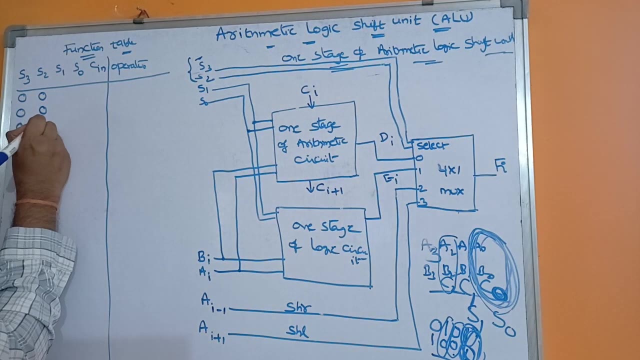 operation will get performed, Arithmetic operation. So if S3, S2 are 0, 0. Then arithmetic operation will get performed Here. totally, there are 8 arithmetic operations are there. So that is why we have to write 8: 0, 0s. If arithmetic operations are 0, 0. Then arithmetic operations will get. 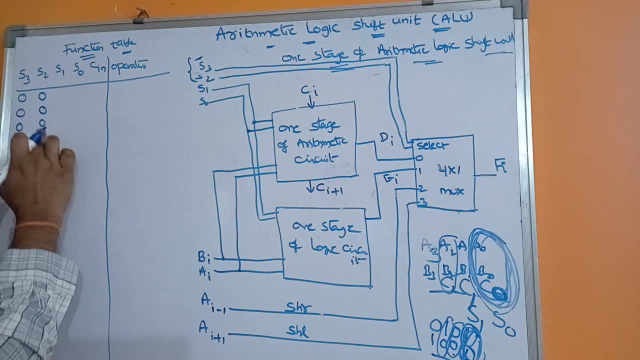 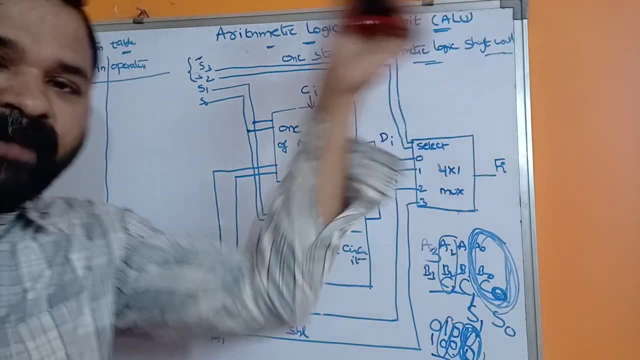 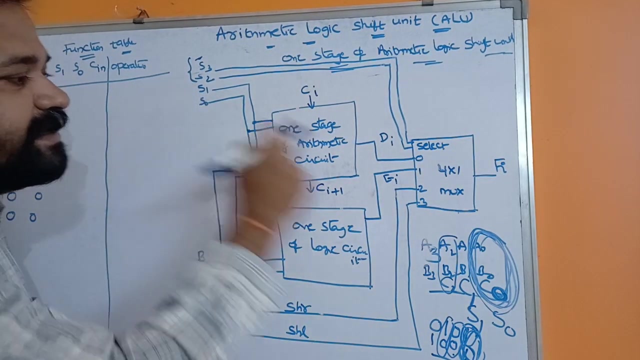 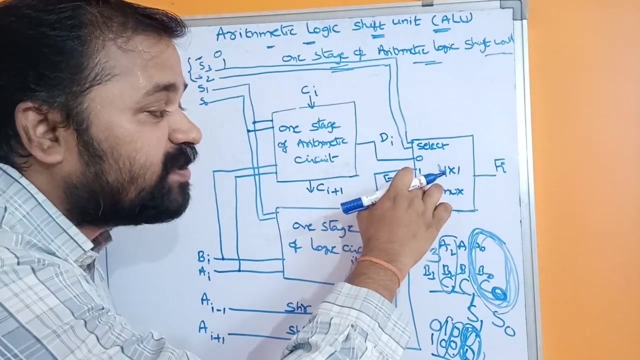 performed: 1,, 2,, 3,, 4,, 5,, 6,, 7,, 8.. So we will write all these operations by taking arithmetic provided by the logic circuit diagram. Next, If the selection inputs, If S3, S2, are 0, 1. Then what is going to happen? This 1 data input will be selected. 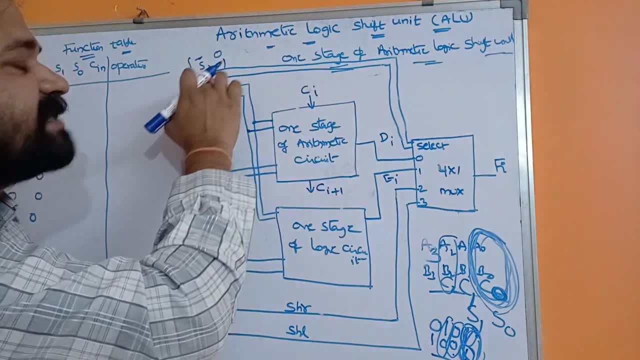 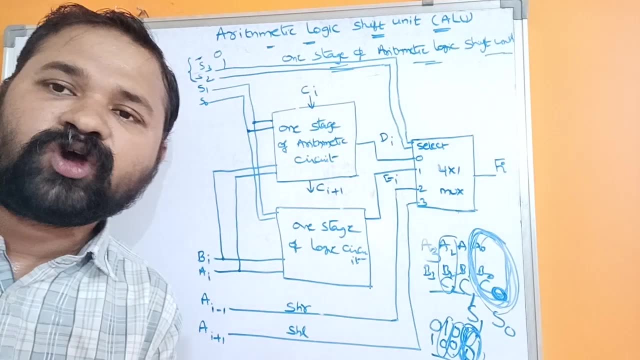 What is the 1 data input, the output of this logic circuit. So that means wenn the operating inputs are 0,1, then logical micro operations will getノ performed. Totally there are 4 logic micro operations are there, So 0, 1.. So you need to Hog. 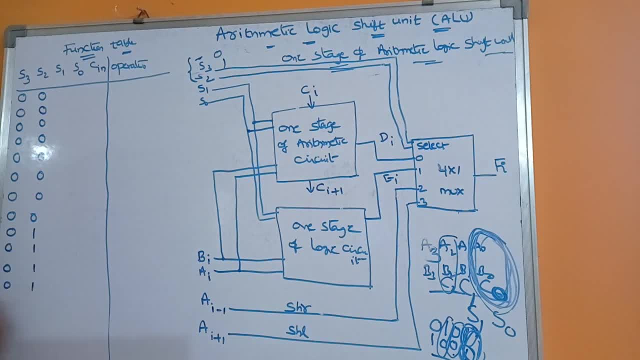 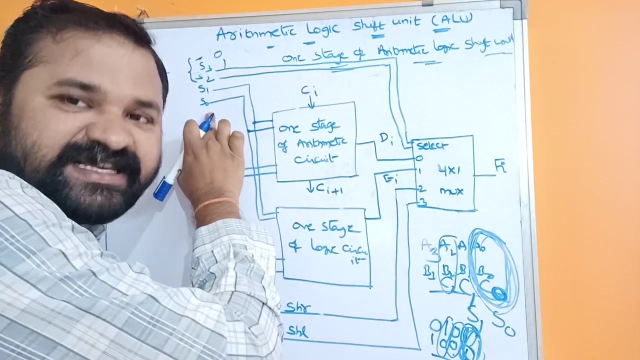 four logic micro operations: zero one, zero one. okay, let us write the logic micro operations. so if the selection if he has three, s two or zero one, then logic micro operations will gets performed next. this logic circuit is controlled by s 1 and s naught. if s 1 and s naught are 0: 0. 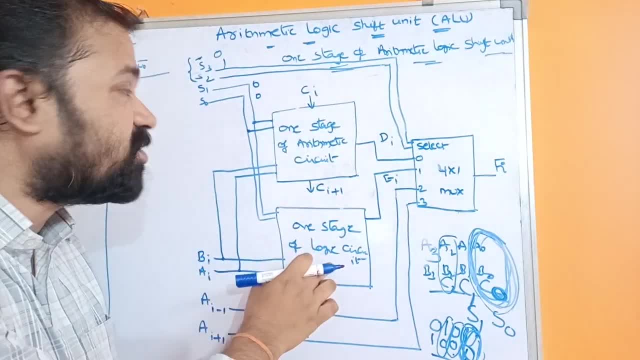 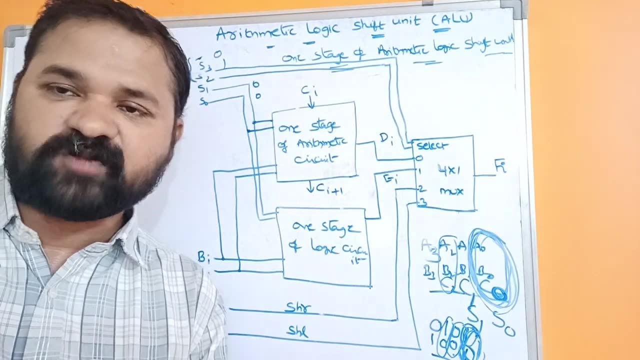 then perform under operation. if s 1 and s naught is 0: 1, then perform r operation. if s 1 s naught r 1: 0, then perform exclusive r operation. if s 1 and s naught are 1: 1, then perform complement. 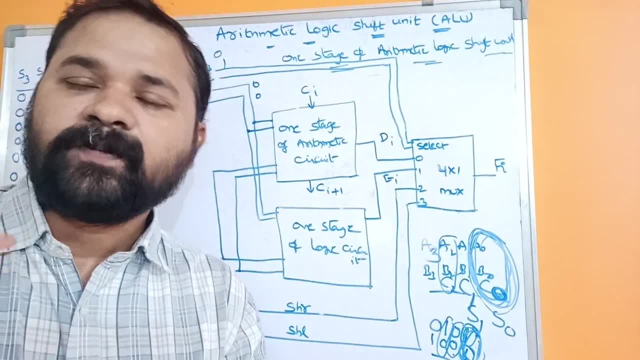 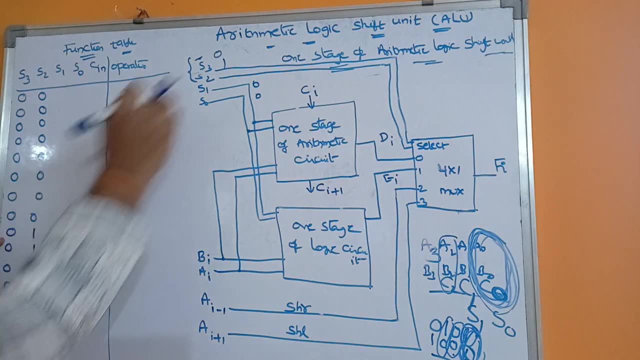 operation. these four are the simple logic micro operations. by using these operations we can implement any other operation. okay, so let us write those operations: s 3, s 2, 0. 1 means logical operations will gets performed. so what are s 1 and s naught? if s 1 and s naught are 0, 0, then which? 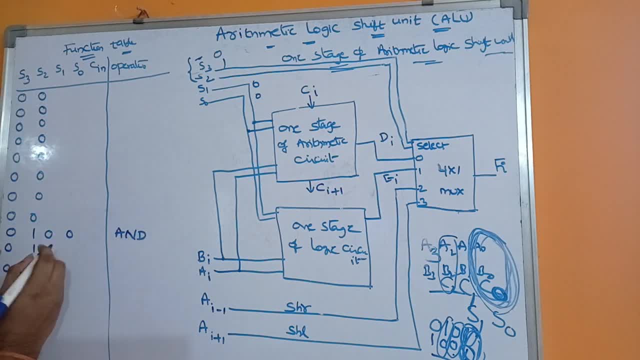 operation will be performed. under operation will be performed, whereas if s 1 and s naught are 0, 1, then r operation will gets performed, 1, 0, then xr operation will gets performed. next, 1. 1 means complement operation will gets performed. okay, next, what is carry value in order to perform? 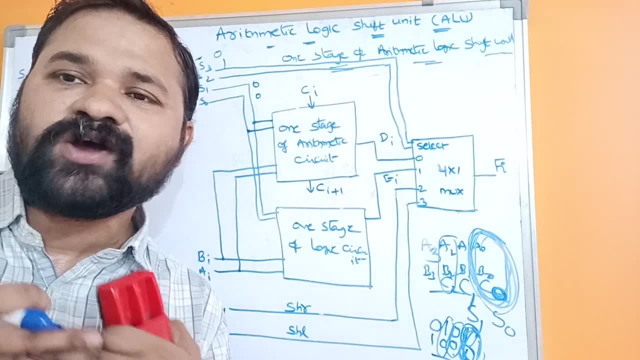 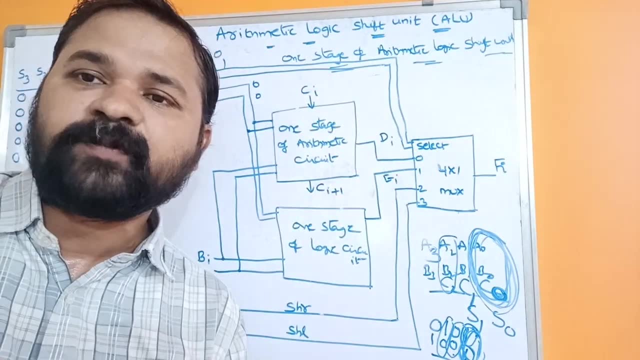 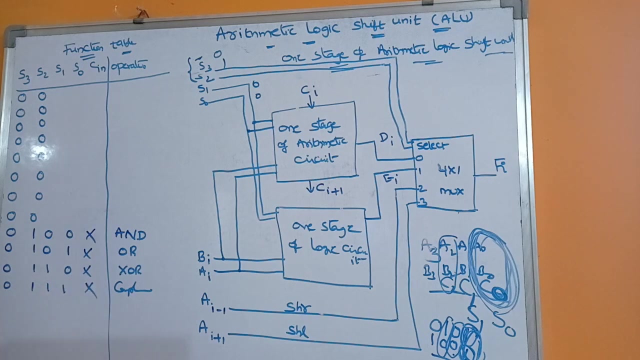 operations. on the logical micro operations, there is no need of any carry. carry is needed only while performing the arithmetic operations. so just use into mark. that into mark represents don't care means we are not using any carry. okay, next, if s, 3, s, 2, r, 1, 0, then which micro operation will gets? 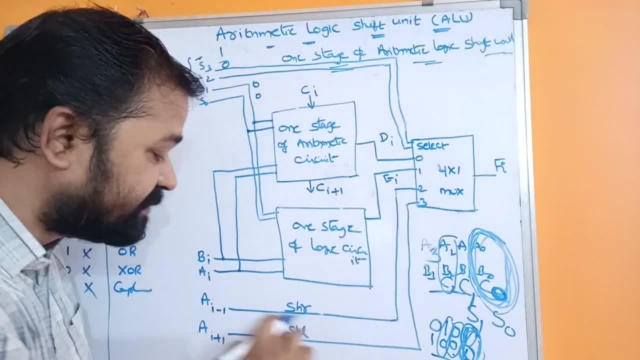 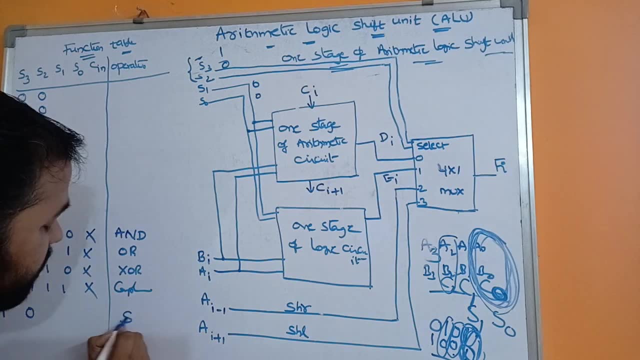 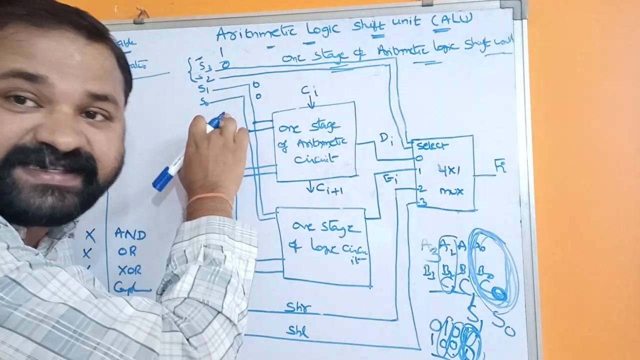 performed this, two data input will be selected. two is getting data from shift right operation. so if s 3 and s 2 are 1: 0, then shift right micro operation will gets performed here. in order to perform the shift right micro operation, there is no need of the selection inputs. 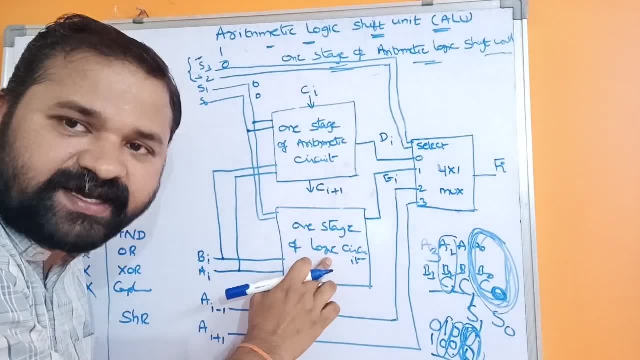 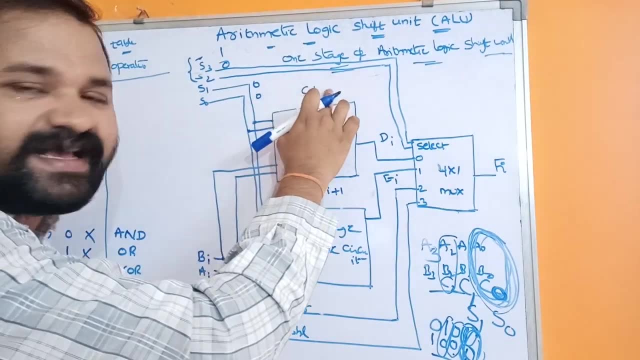 these selection inputs controls only arithmetic operations and logic micro operations. okay, while performing shift right and shift left, there is no need of this s 1 and s 2 as well, as there is no need of this can. so right don't gets, so this don't get. 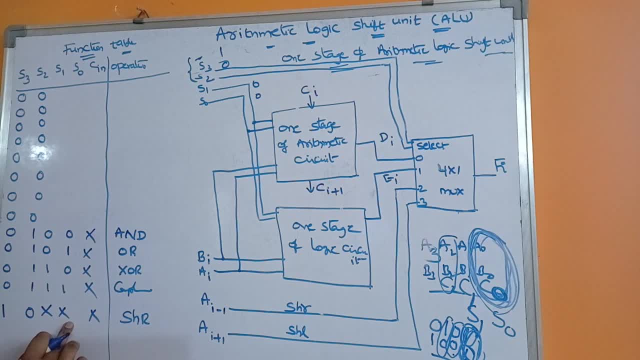 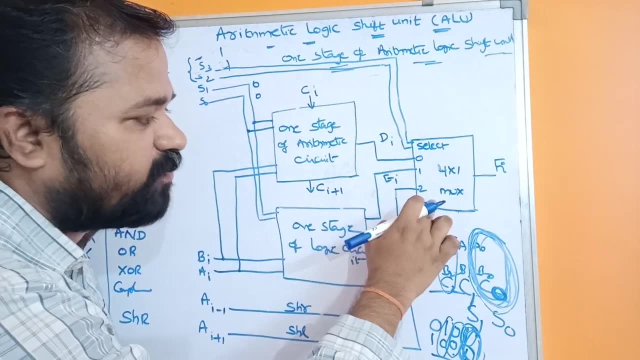 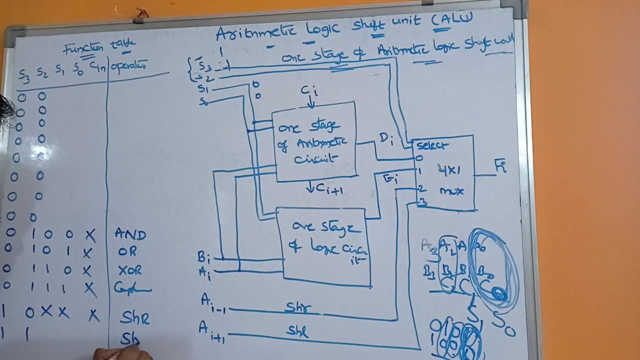 specifies that we are not using selection, these two selection inputs as well as this carry value. next, if s 3, s 2, r, 1, 1, then which operation we are performing? input 3 data will be selected. so that means we are performing shift to left operation. shift to left operation. okay so. 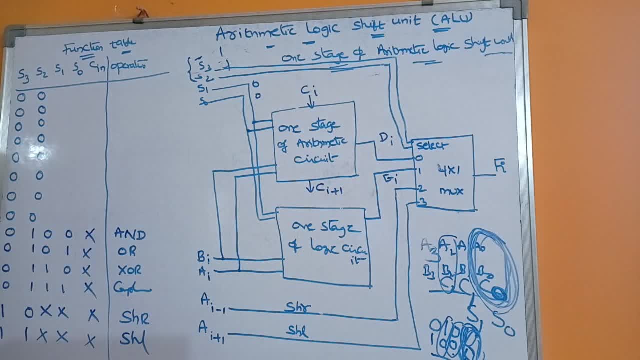 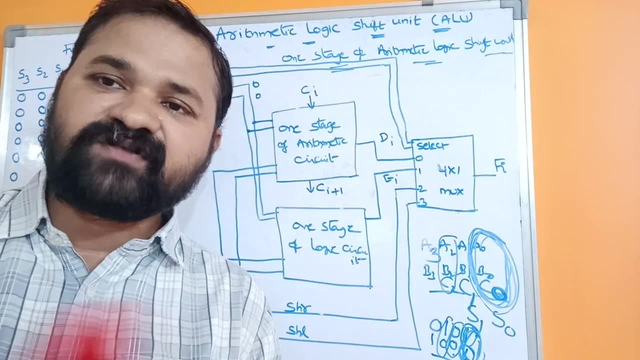 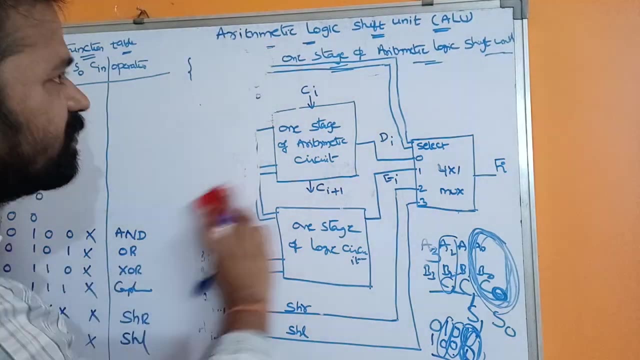 just use don't gets. that means we are not using s 1, s, naught and this input carry value. so with this, logical micro operations are over, as well as shift micro operations are over. so now let's see about arithmetic micro operations. so already we have seen arithmetic micro operations circuit. 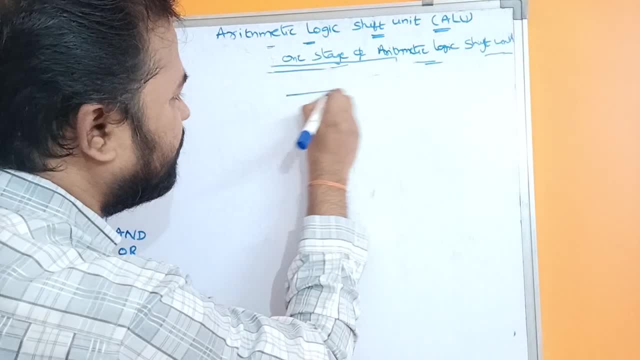 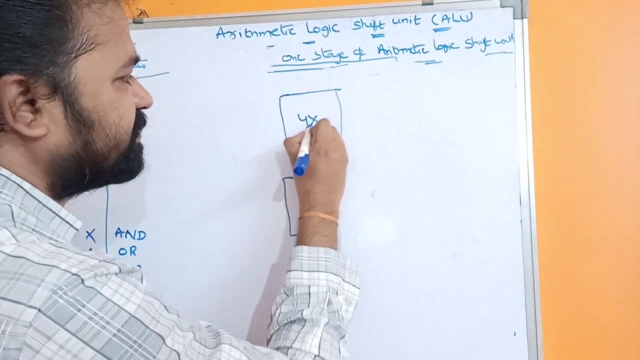 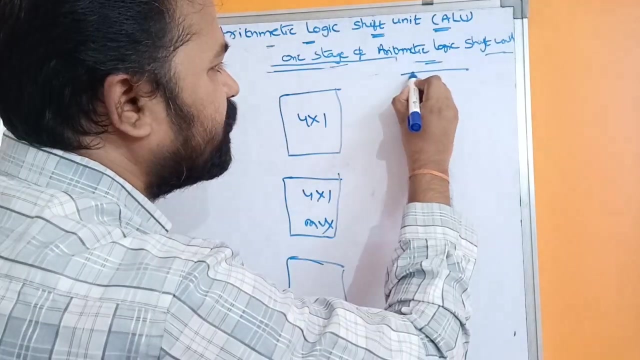 but here we have to write those values also. so for that let us see in brief: so we have let we have two multiplexers, so 4 by 1 multiplexer, 4 by 1 multiplexer. so likewise generally we will take four multiplexers. next, in order to perform the addition, we use some fully added. so likewise we. 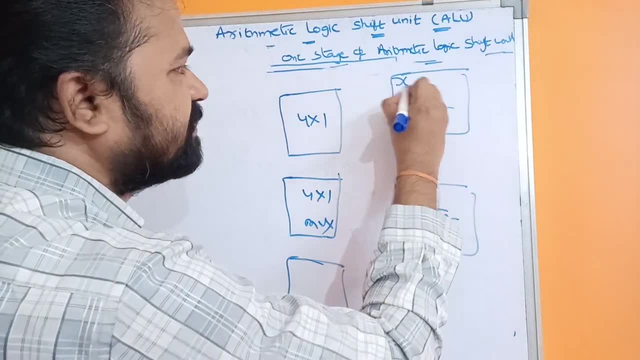 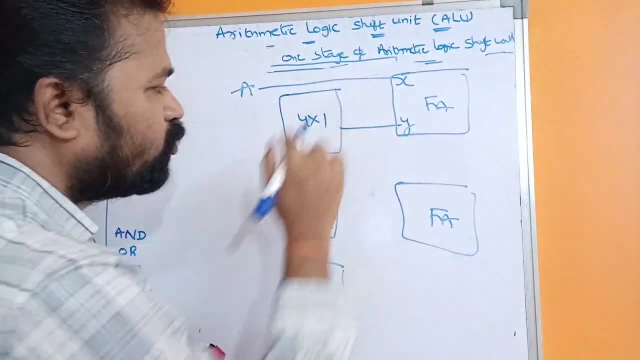 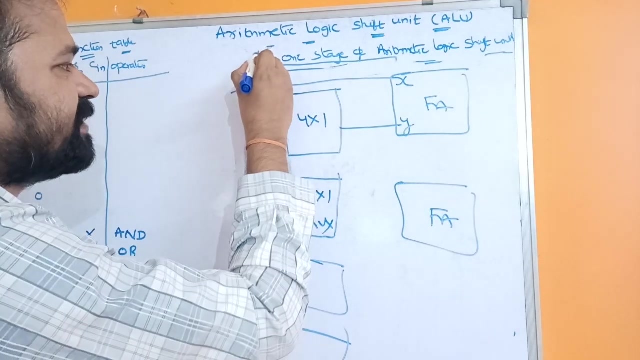 use fully added. so this is nothing but x. this is nothing but y. here, x gets data from register a. y gets data from output of the multiplexer. s 1 and s naught are nothing but selection inputs of the multiplexer. s 1 and s naught are nothing. but these are nothing but selection inputs of the multiplexer. 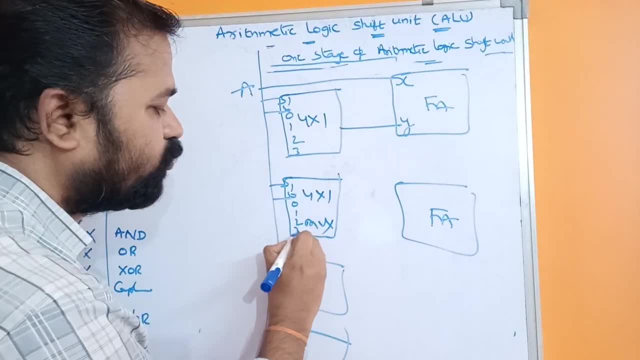 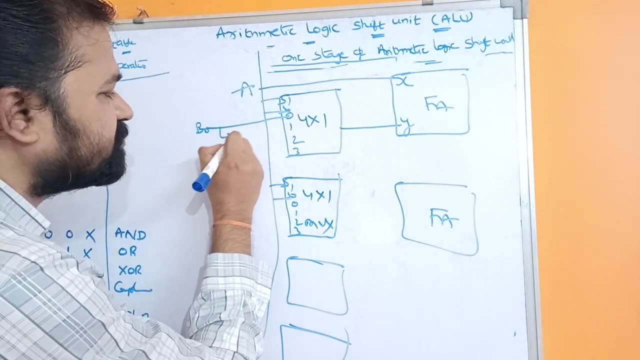 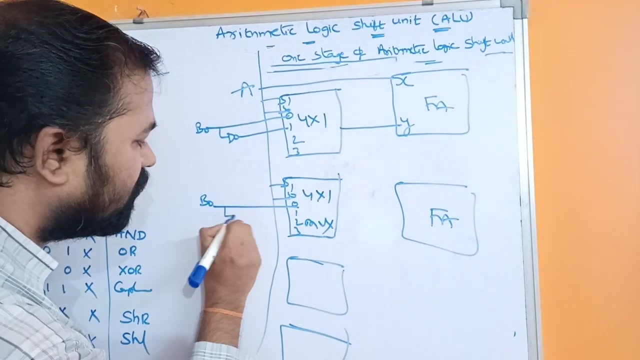 so here 4 by 1 multiplexer means we have 4 inputs. 0 input receives data from register b, whereas one input receives data from complement of b. so likewise, zero input receives data from b, one input receives data from complement of b. so likewise for the remaining two multiflexers also. 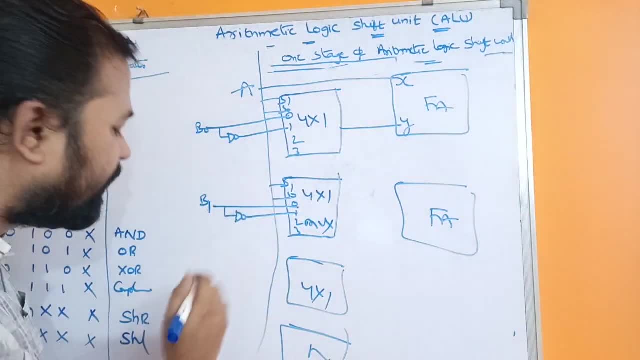 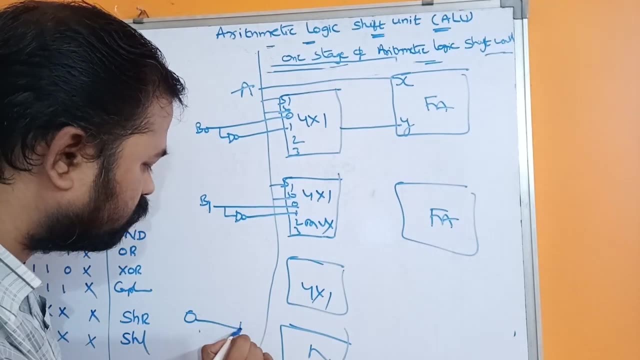 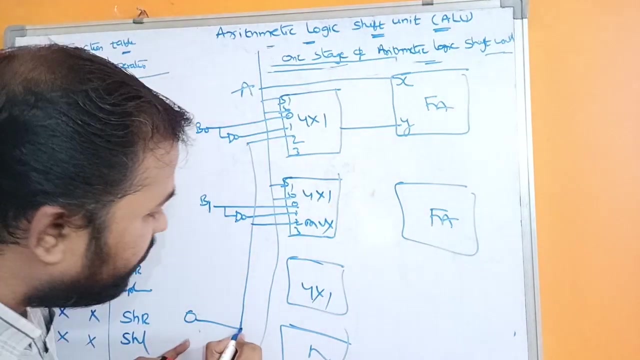 set. so let it be some b soнымas: 1. next, this 2 and 3 gets data from 0. this 2 and 3 gets data from 0. this 2 data input gets data from 0, whereas 3 data input gets data from 1. 0 complement means what 1? 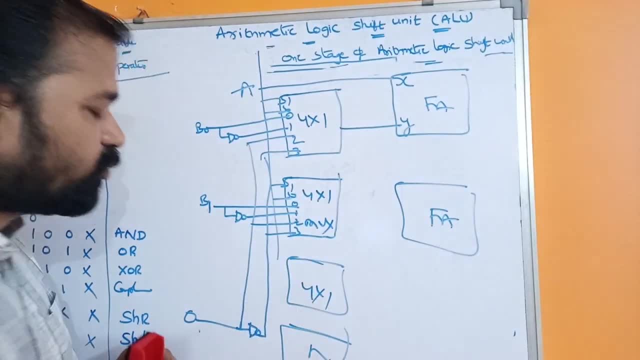 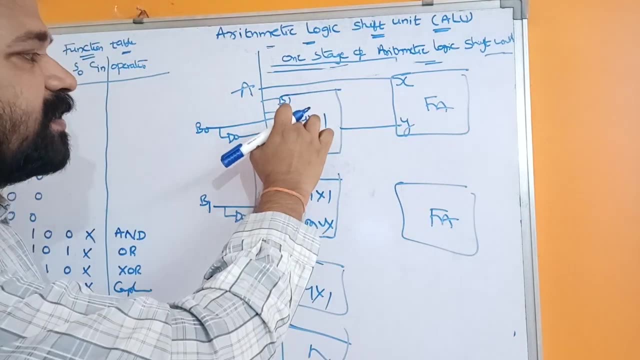 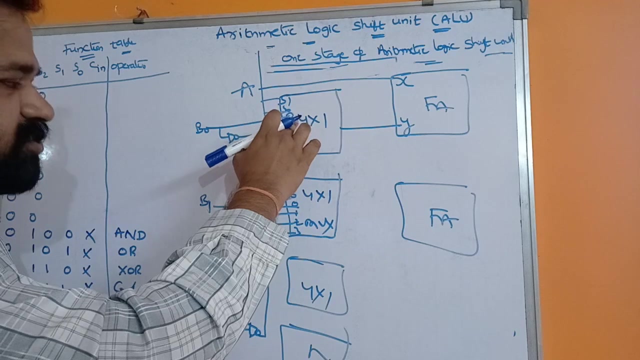 so here the point is very, very simple. this is nothing but arithmetic circuit. so here we have four selection in four. two selection inputs- s1 and s0- are nothing but selection inputs. 0, 1, 2, 3 are nothing but data inputs. here, 0 is data input, 0 is getting data. 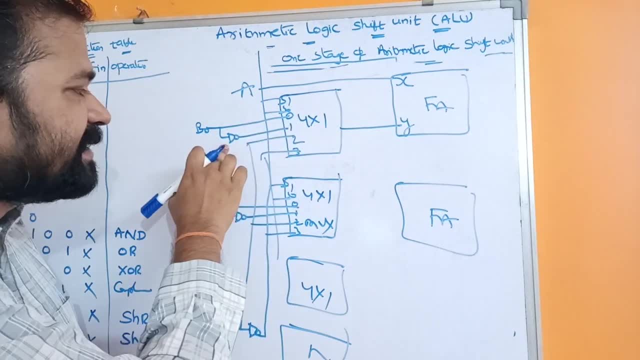 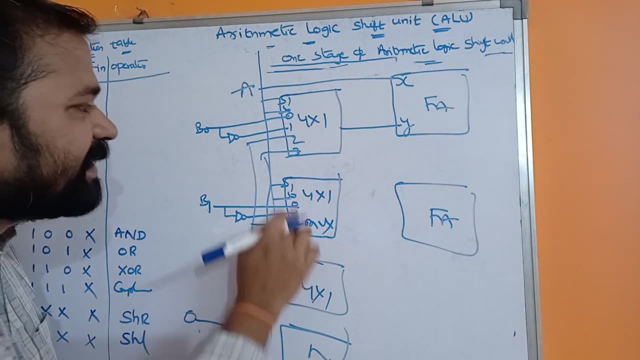 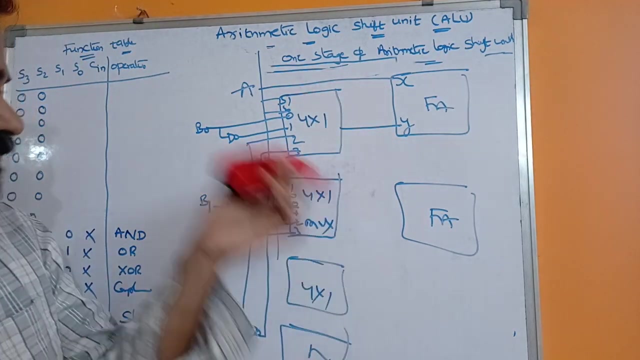 from register b. next data input 1 is getting data from complement of b. next to 2 data input is getting data from 0. here, Three data input is getting data from complement of 0. Complement of 0 means 1.. Now, based on this, we have to perform the operations. 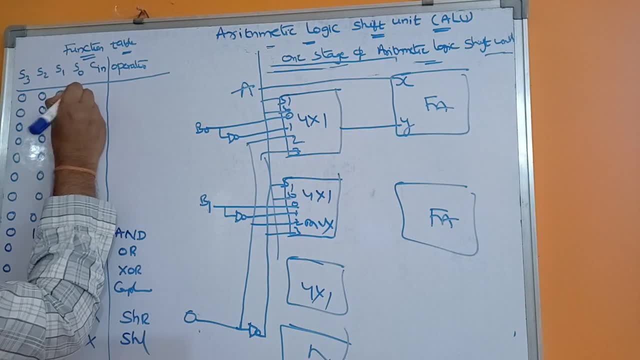 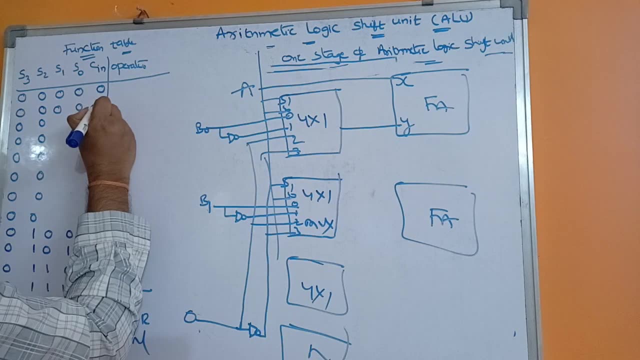 Let us assume that the selection inputs are 0, 0.. Selection inputs are 0, 0. If the selection let, the selection inputs are 0. And here the carry value may be either 0 or 1. So here a carry will be passed to the corresponding fully added. 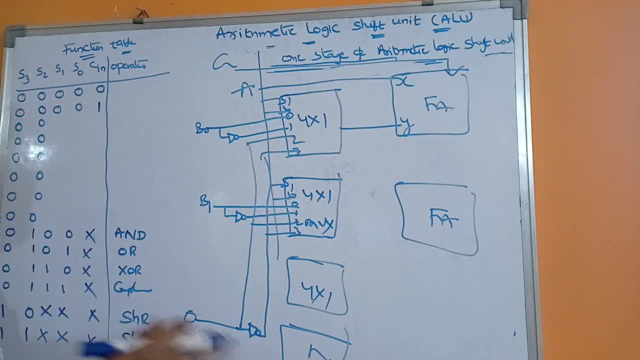 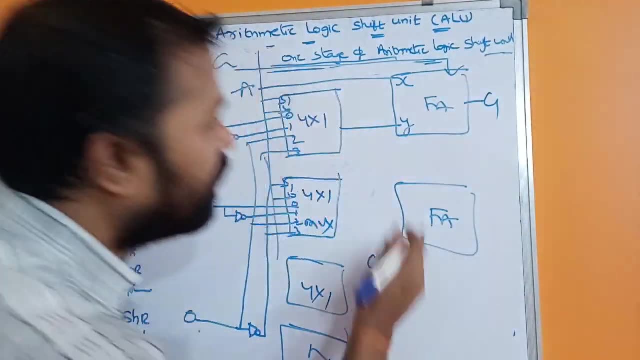 So carry value may be either 0 or 1.. Now let us see what is the operation Which gets performed. Let this output is denoted by some g, So this g is equal to. Here the formula for the output is: 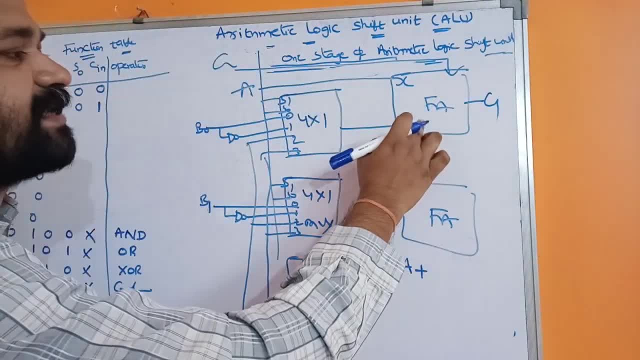 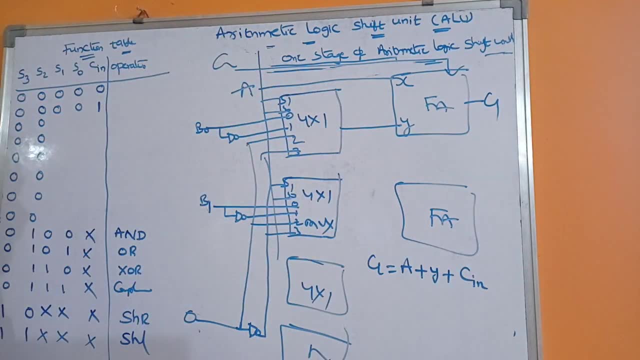 X is getting data from a, a plus Next. y means directly: it is getting data from output of the multiplier y plus e, i, u. This is nothing but input carry. So what is a here? a means it is directly getting the data. 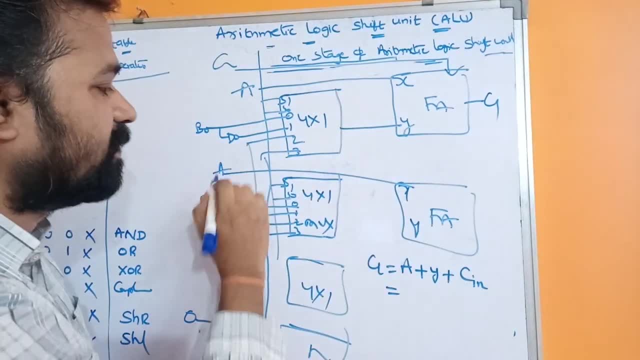 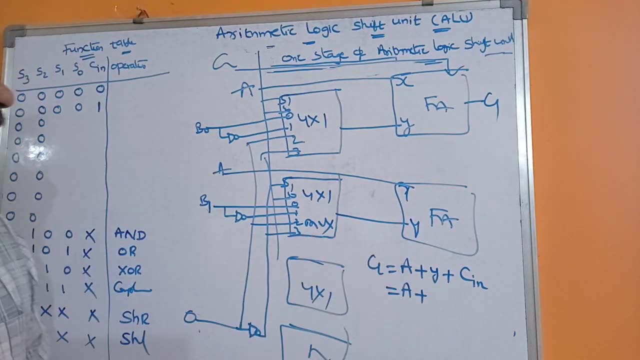 Here also we have some x and y. X receives data from a, y receives data from output of the multiplier. So here a is getting data directly. Next, what is y here? So y means output of the multiplier. So output of the multiplier. 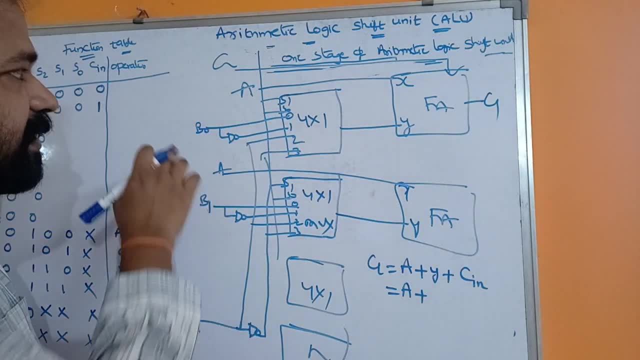 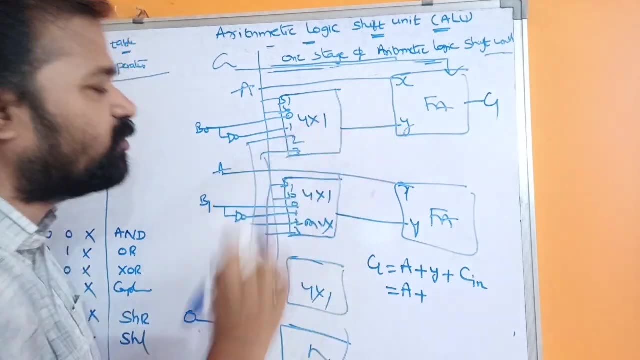 Here. what are the selection inputs? 0, 0 are the selection inputs. If 0, 0 are the selection inputs, Then 0 data input data will be selected And this data will be produced as the output. Here, 0 is getting data from which register. 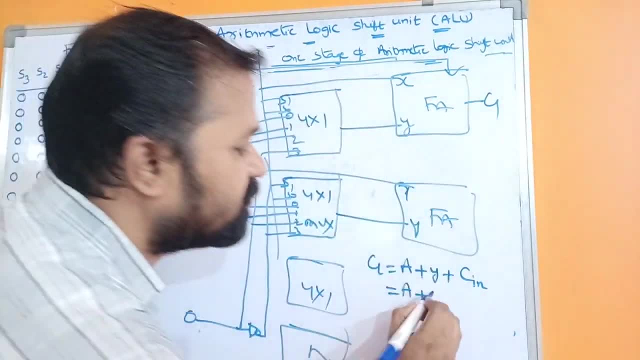 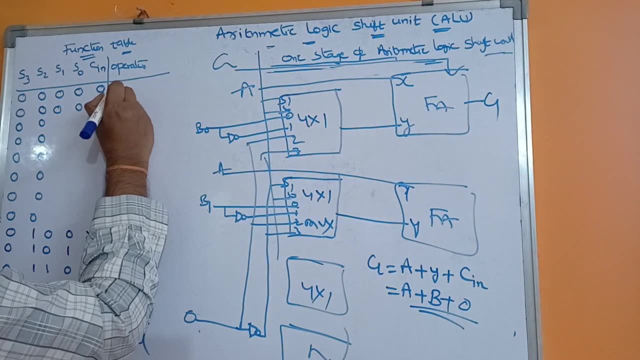 B register. So here y means output of b, So b plus. So first what is carry value? C is nothing but carry value. So that is nothing. but Here the operation is a plus b. a plus b is nothing, but what. 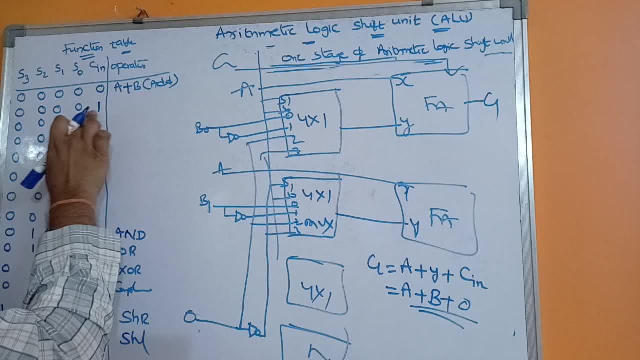 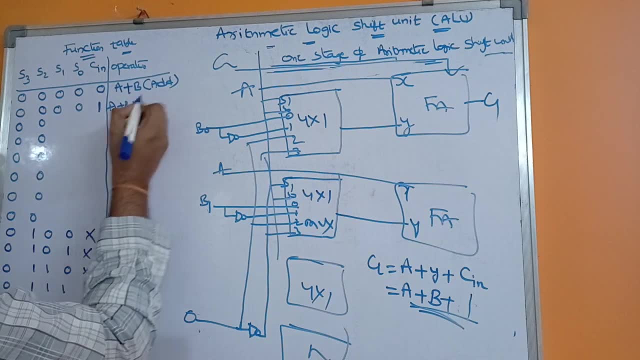 Addition operation. we are performing Next, same selection inputs, But the carry value is 1. So here the seeing is 1.. So the operation which we are performing is a plus b plus 1. So this is nothing but addition only. 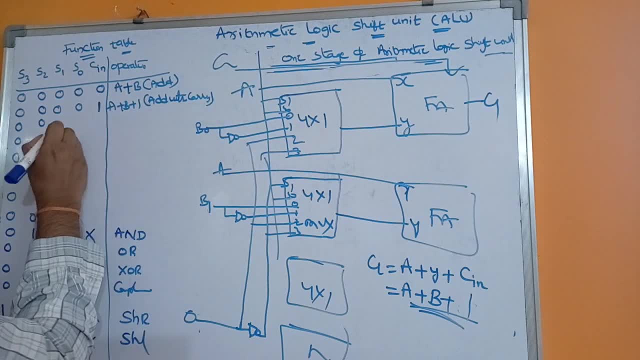 Addition with carry. But here we have 1 here. Next let us take the selection inputs 1, 0.. Here the carry value is 1.. So the carry value may be either 0 or 1.. Now let us calculate here. 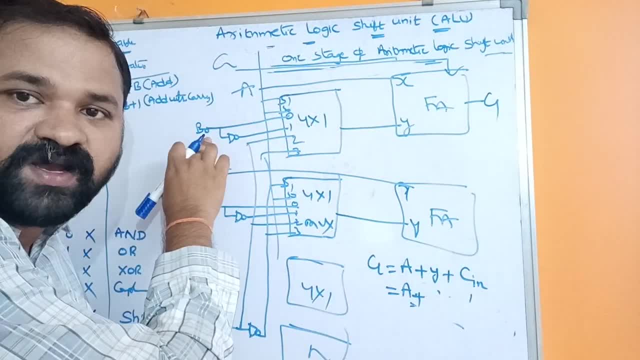 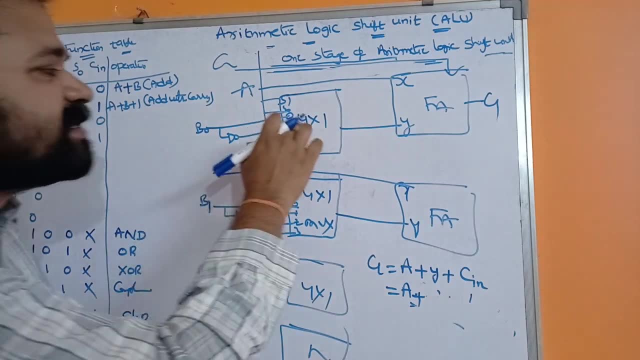 If the selection inputs are 0, 1. Then what will happen? 1 input data will be selected And the data will be passed as input to the y. So what is 1 input data? 1 is getting data from complement of b. 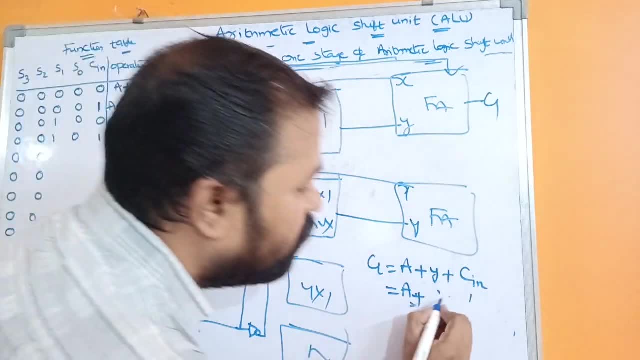 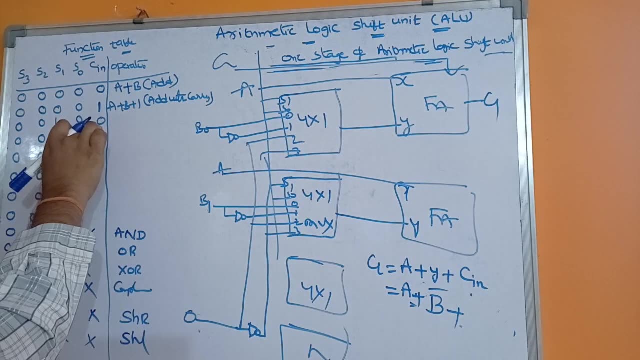 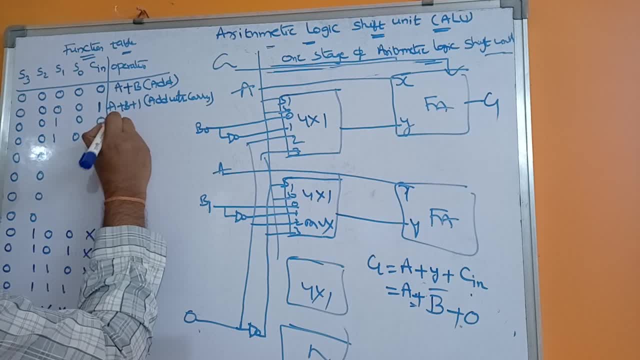 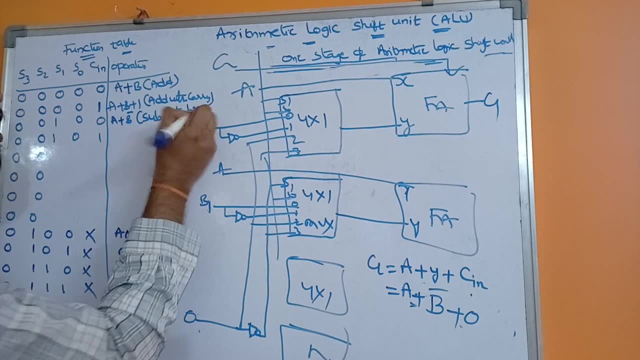 a plus b bar plus 0.. a plus b bar plus 0 is nothing but a plus b bar. This operation is called as subtraction with borrow. This operation is called as subtraction with borrow. Next one: carry value is 1.. So carry value is 1.. 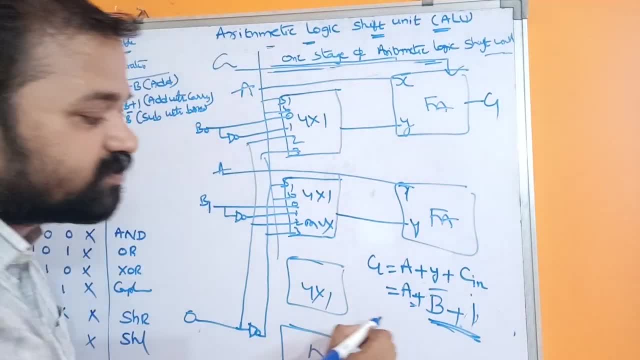 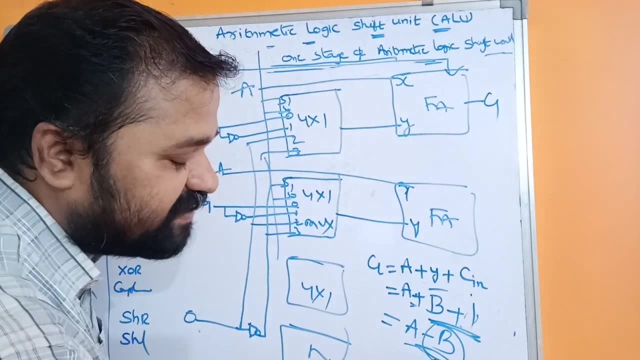 a plus b, bar plus 1.. This is nothing but 2's complement of b. So this operation is nothing but subtraction operation. We know how to subtract two binary numbers by adding 2's complement of 2nd register to 1st register. 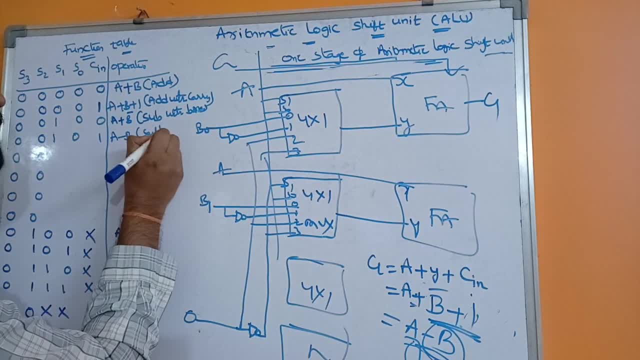 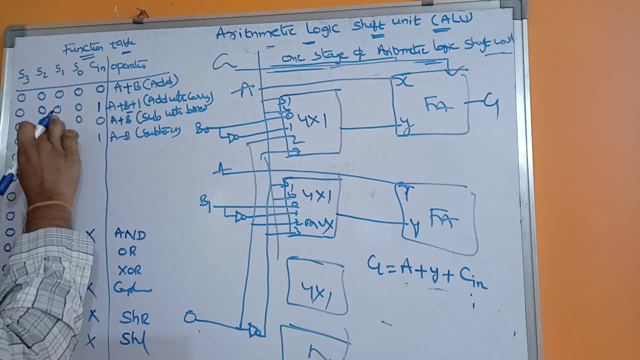 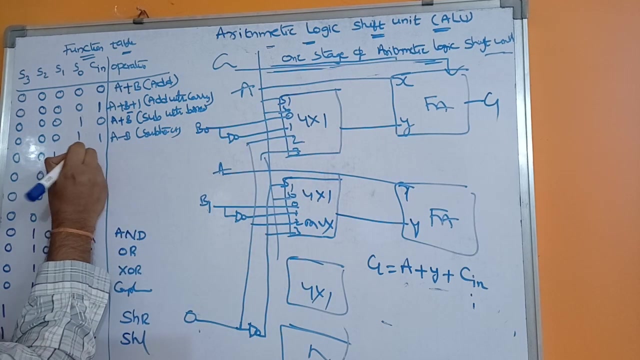 So this is nothing but a minus b. so what is a minus b? a minus b is nothing but subtraction operation. now let us consider about the next situation. that is zero. zero is lower. i'm sorry, this is zero one, this is zero one. zero one means one data input will be selected. so next combination: one zero, one, zero. here the carry. 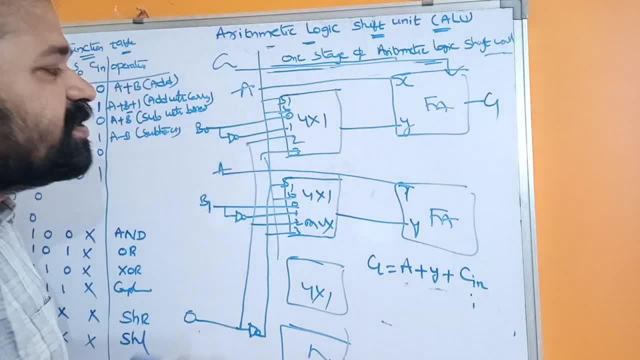 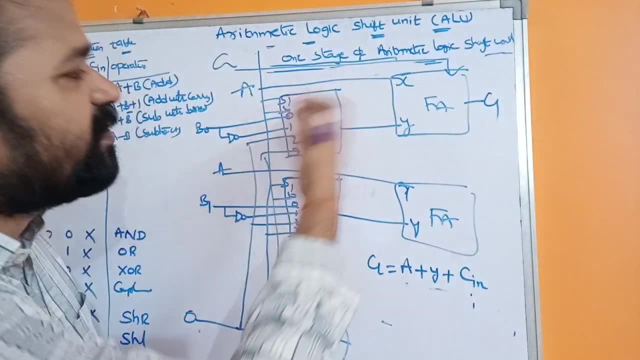 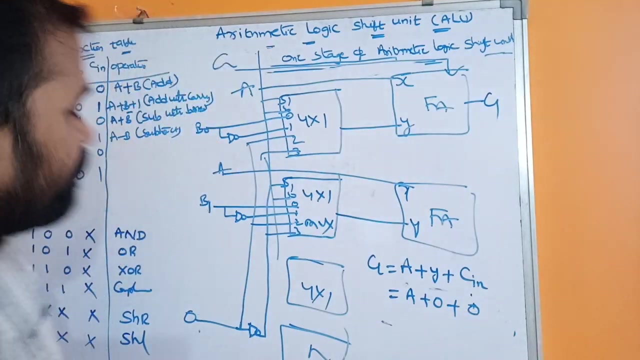 values may be either zero or one. so if one zero, if the selection inputs are one zero, then two data input will be selected here. two is getting data from zero. so the zero will be passed as input to the pi. so a plus zero, plus what is the carry value? zero? that is nothing but a. so a means what here? 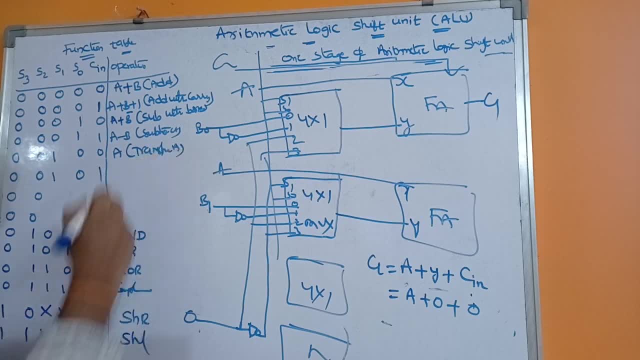 the operation is transfer operation, so transfer a. next: carry value is one, carry value is one, so that means this is nothing but increment operation, so increment a. next, the last combination: one one. so here the carry value may be either zero or one. okay, now let's see here: okay, if the inputs are one one. 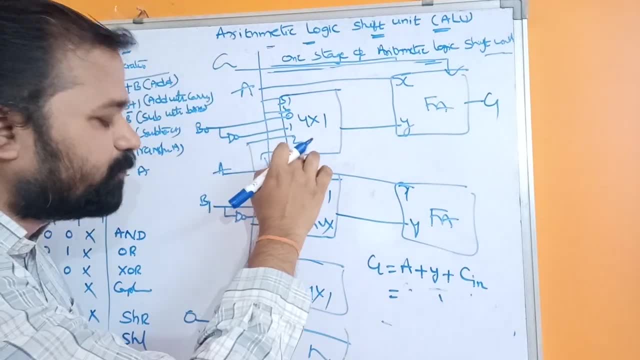 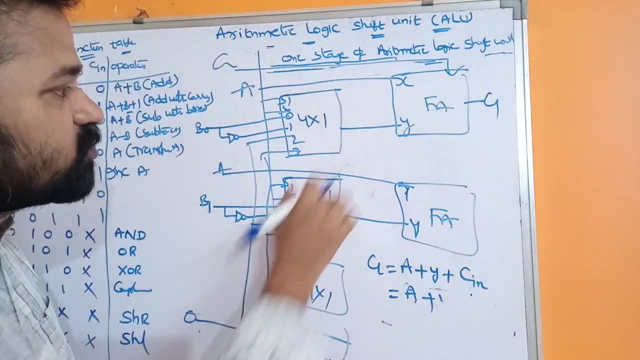 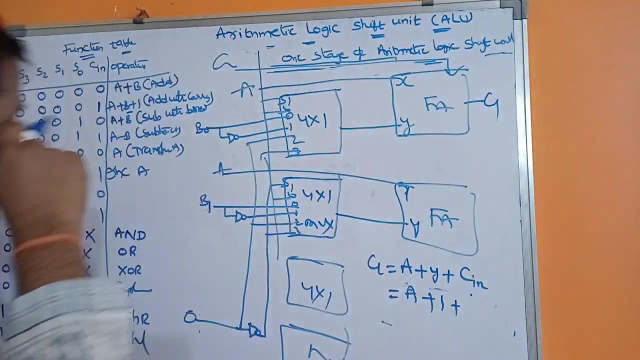 then three data input will be selected. what is three data input? it is getting data from complement of zero. that is nothing but one. so a plus. it is getting data from one, so we will get all ones. if the if there are four resistors, then we will get four ones. so a plus one plus. what is the carry? 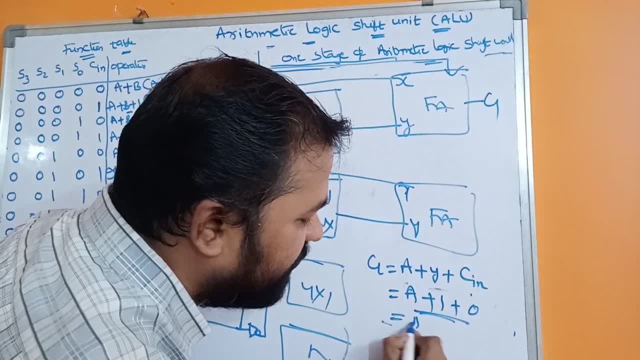 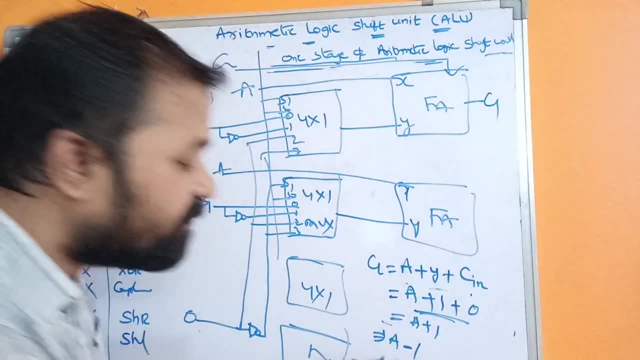 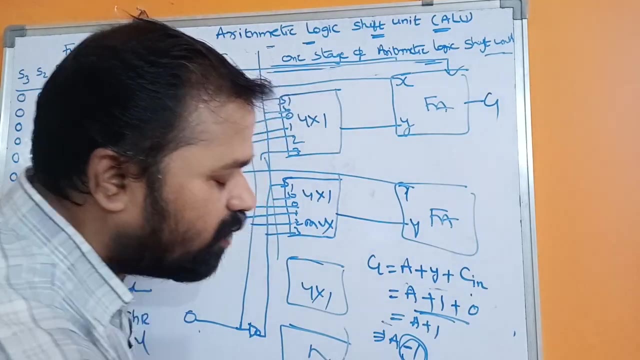 value. here, zero is the carry value. so this is nothing but a plus one. a plus one is nothing, but we are performing the operation a minus one. why? because what is a minus one? a minus one means we have to calculate two's complement of one, and that should be added to a. so how to calculate two's complement of one? for that? 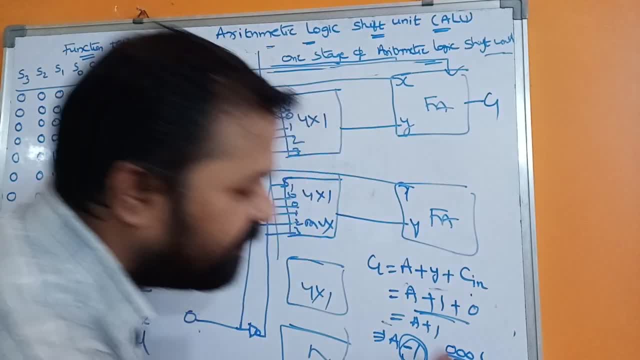 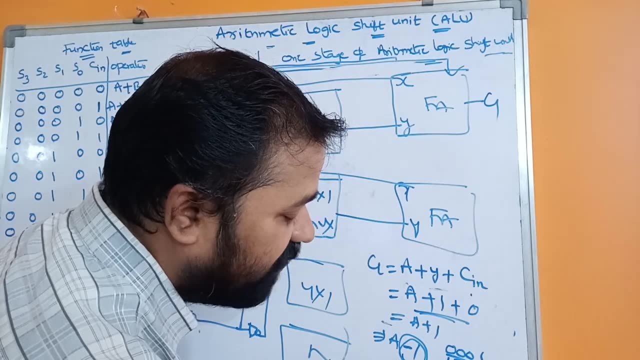 first we have to represent one in binding notation- three zero one. next to calculate two's complement. so two's complement means first we have to calculate one's complement, so three, one, zero. next we have to add one, so all ones here. what we are doing here we are adding four ones if there are. 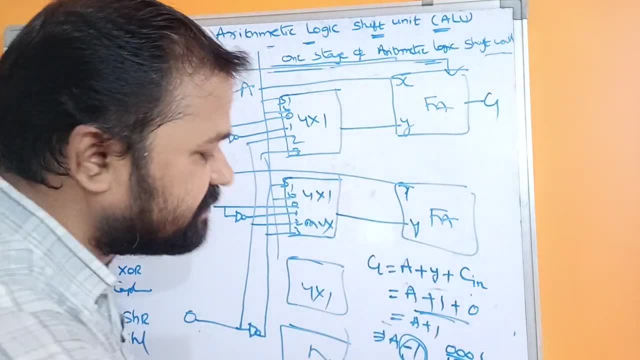 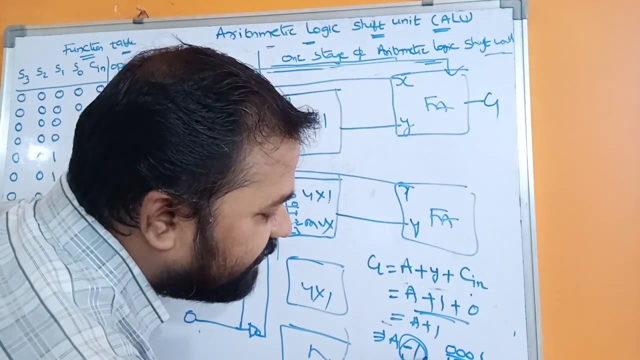 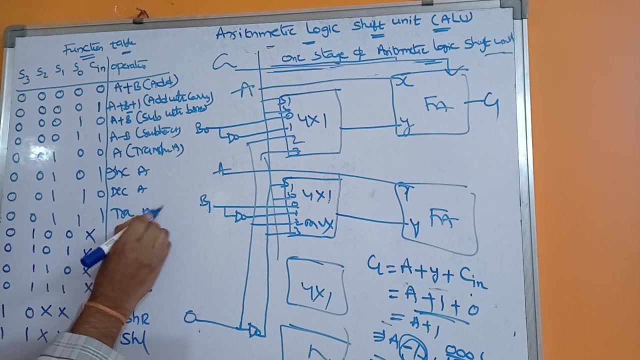 four bits, then we have to add those four bits. so this is nothing but a minus one. a minus one means what decrement here? next we have to add the carry. so if we add carry to a minus one, then what is the output? a minus one plus one. that is nothing but a. so this is nothing but transfer a operation. 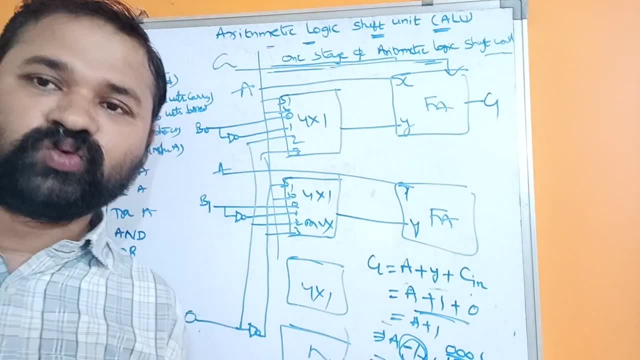 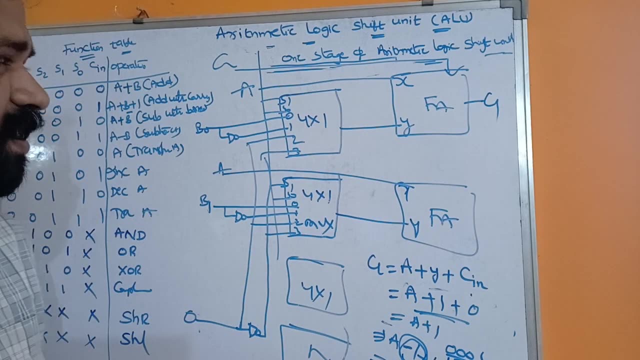 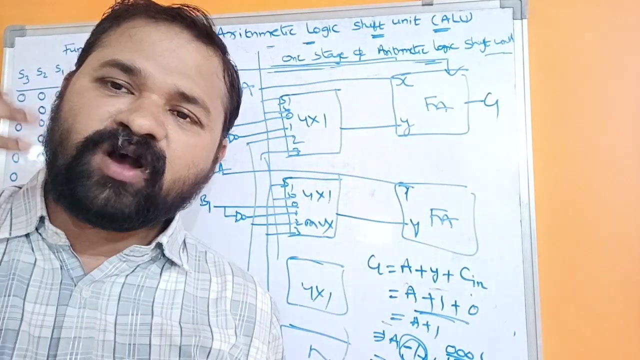 so these are the eight plus four plus two, so eight arithmetic operations, four logic micro operations and two shift operations. we can perform all those although these operations with the help of this arithmetic logic shift unit. so by using these operations we can perform the remaining all other operations. 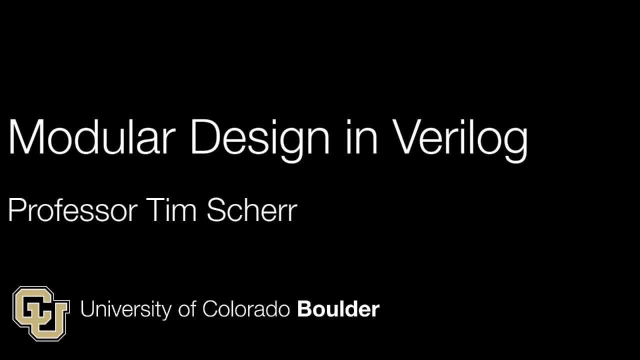 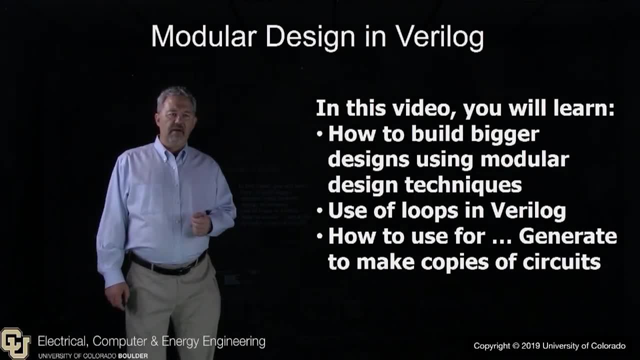 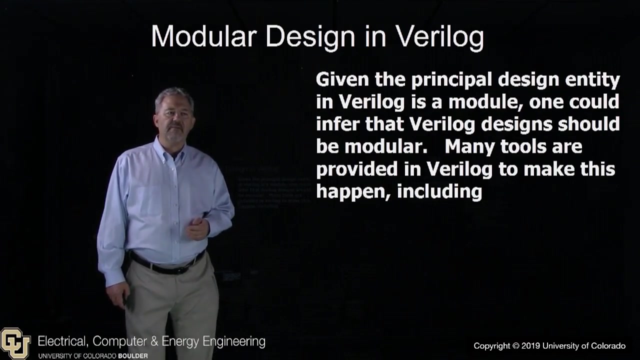 In this video you will learn how to build bigger designs using modular design techniques, the use of loops in Verilog and how to use 4Generate to make copies of circuits. Given the principal design entity in Verilog is a module, one would infer that Verilog designs should be modular.